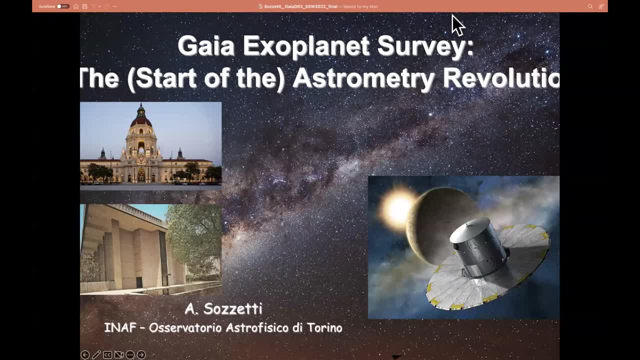 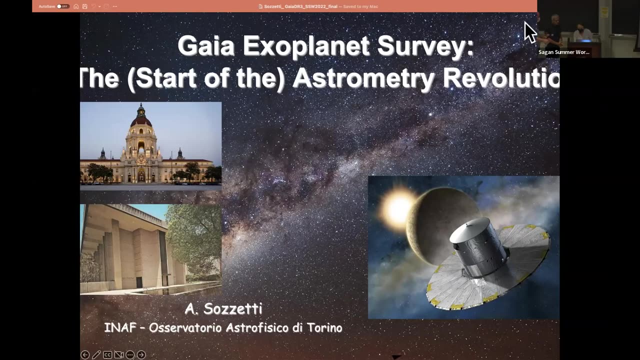 about the Gaia Exoplanet Survey, the Astrometry Revolution. You have 50 minutes and 10 minutes for questions. Well, good morning everyone. In case I have tried to avoid using entirely the very last corners on the left and the right of the slides, 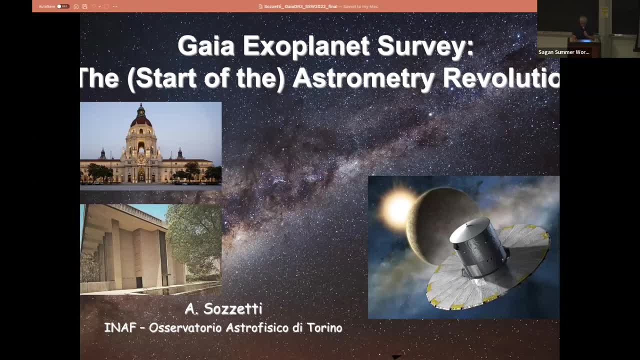 if something gets cut, I'll try to tell you in words. So I have the pleasure to introduce you a little bit more to the gist of Gaia's Astrometry and Exoplanets. Before I do that, I think it is necessary for me to spend a few words about a colleague and a friend. 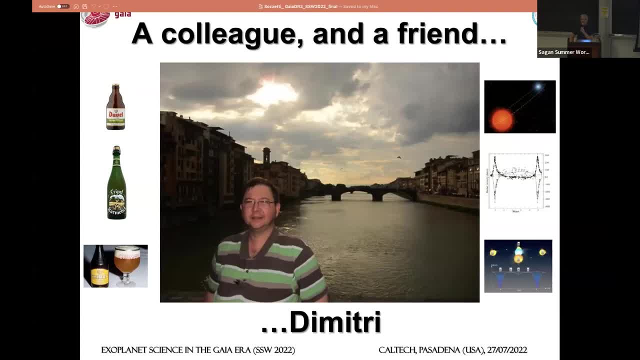 who should have actually most likely been in my place today. He's not with us anymore. He was a wonderful person, a foremost expert in binary astronomy, a fantastic expert. of the most important thing, he is a mastermind behind the full architecture of the data processing pipeline. 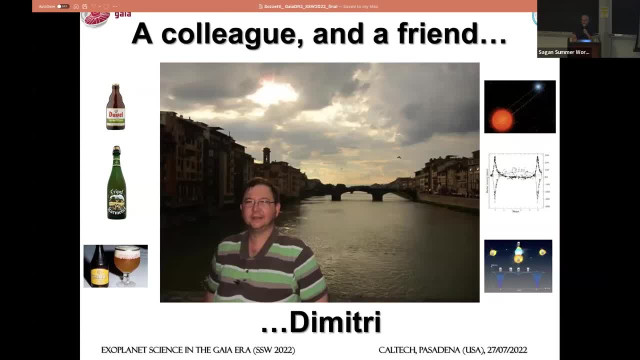 that has produced the results that have populated Gaia DR3. just a little more than a month ago, You should have seen these numbers and it should be here to commend them. in my place now, i have had the pleasure to be spared some of the nitty-gritty of astrometry thanks to the excellent introductory. 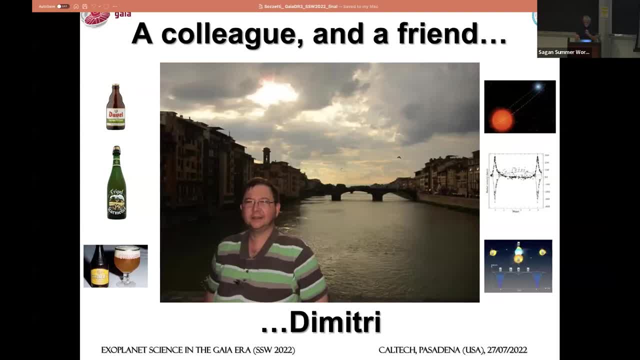 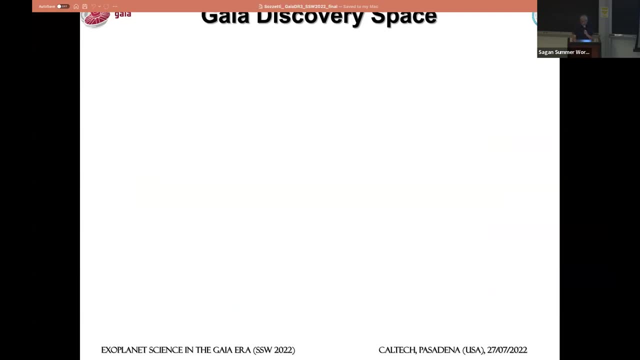 talks from michael perriman and toleri at the beginning of the workshop. so we'll plant right away into some of the main gist and i will start with something that some of you may have already seen times and again, but it's good to get a reminder. there is a out, there an expectation. 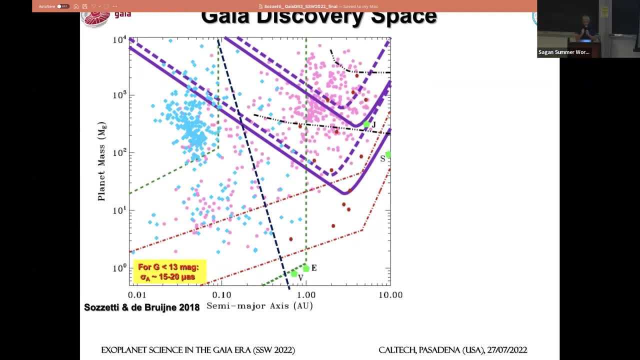 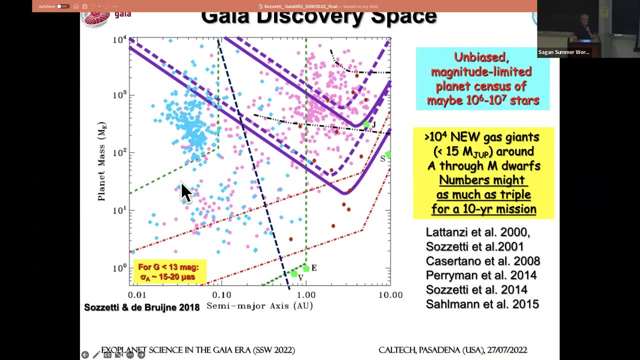 for gaia to find planets and we can use this tool- planetary mass orbital semi-major axis diagram- to figure out gaia can do. in this diagram, i would like you to focus on the proper curves. these are coming in two fashions: one dotted, one solid. they correspond to gaia sensitivity. 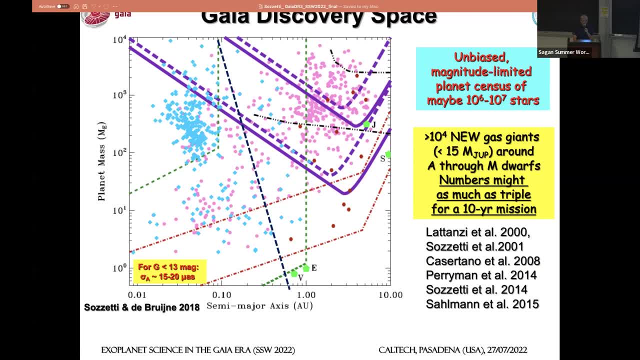 curves for objects, let's say, at the distance of 150 parsecs or so, the nearest star formation regions, towers or ego. or instead, corresponding to the probability of detecting planets around one of the nearest stars to the sun, maybe 20 parsecs or so. these are the ones below. 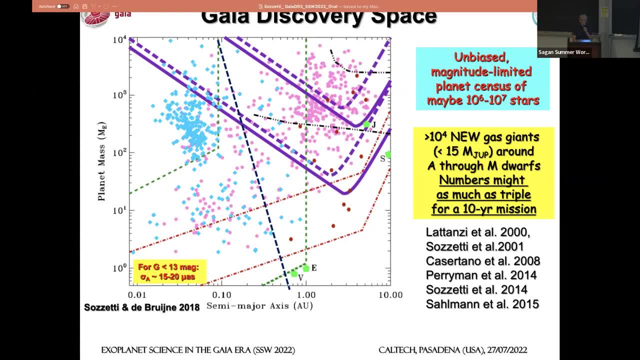 the dotted is the one corresponding to an estimated sensitivity for a nominal five mission duration of the operations, and this one instead corresponds to a full, fully extended 10-year mission of gaia. as you understand from the diagram, there is essentially a region of the parameter space that is 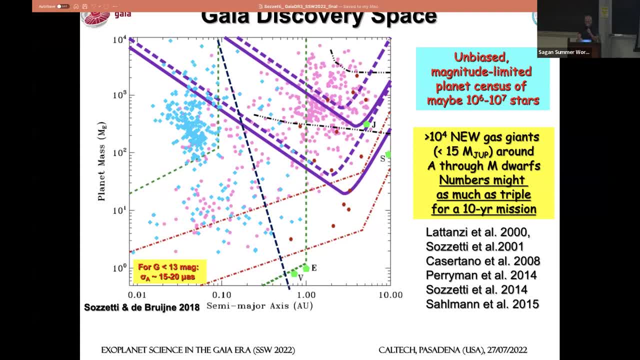 gaia, which is massive objects, giant planetary companions, on orbital uh separations approximately starting at a significant fraction of an astronomical unit all the way out to several astronomical units. this, as far as, for example, transit work or extreme precision- rather velocity work- from the ground is concerned, doesn't seem to be particularly compelling in terms of. 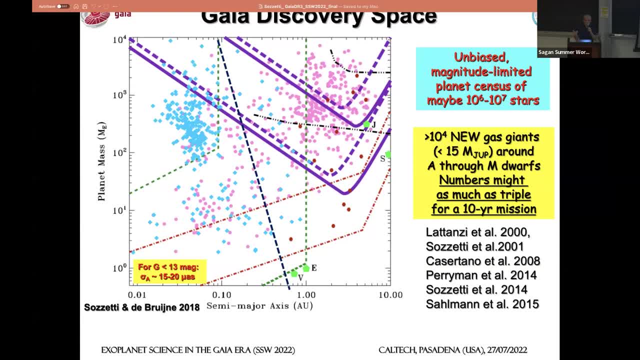 the tractability of companions, because these companions are very well known, they have already been detected, and theJennings are really well known, they are already being detected, and the And some of the frontier work of the field is really aimed at looking at very, very small radius. 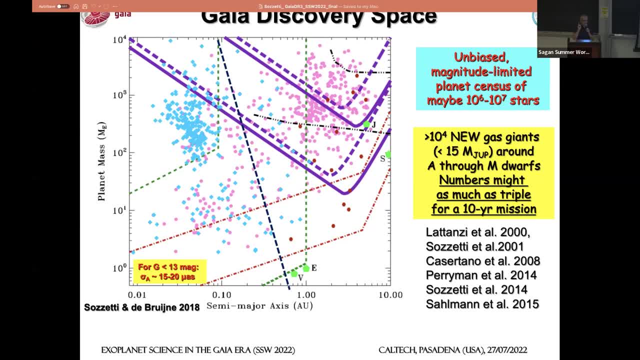 and small mass companions. However, as you can see in this small box over there, the fundamental key point to bring home is that Gaia is expected to find such companions around an extremely large number of stars, And this is the fundamental contribution of the mission. 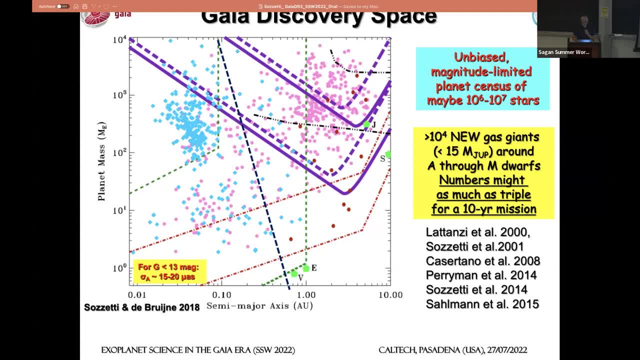 to exoplanetary science. I summarize here a large body of work that has contributed to estimating Gaia sensitivity and finding the number of planets that Gaia can actually uncover, And these numbers come in the thousands, maybe in the tens of thousands and maybe three times more. 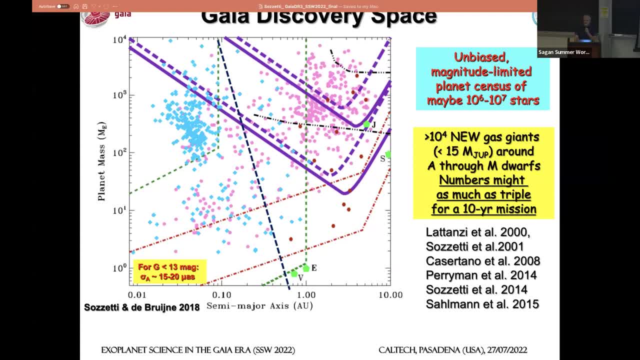 if, as we all hope, a full, extended mission will be able to be carried out. So the bottom line is that you have the possibility to use the Gaia data in perspective to perform planetary system demographics for giant planetary companions. the level of resolution. 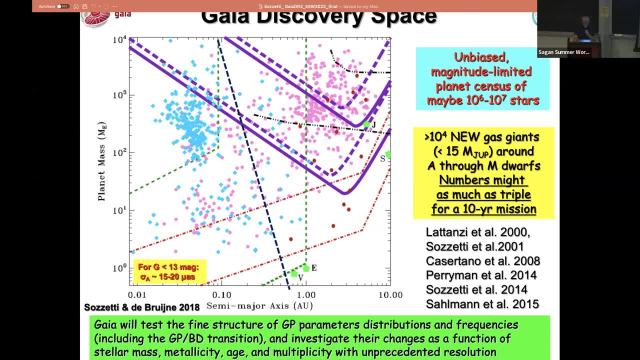 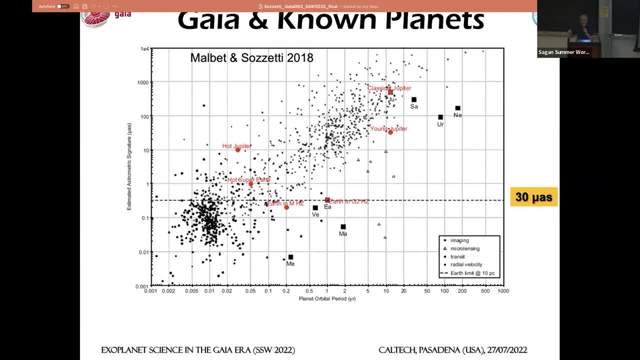 that has never been obtained before. I will briefly touch upon four points that you will see coming back again when we will discuss the outcome of Gaia-3.3.3.3.3.. data release: One first spectacular element of Gaia contribution. 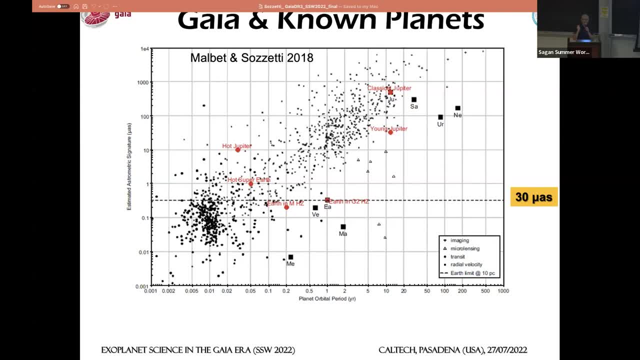 is the possibility of measuring the masses of other velocity planets that have, as you have seen through the initial talks, this ambiguity in the determination of the actual value of the mass companion, in that you can only derive a minimum mass for the object with this technique. 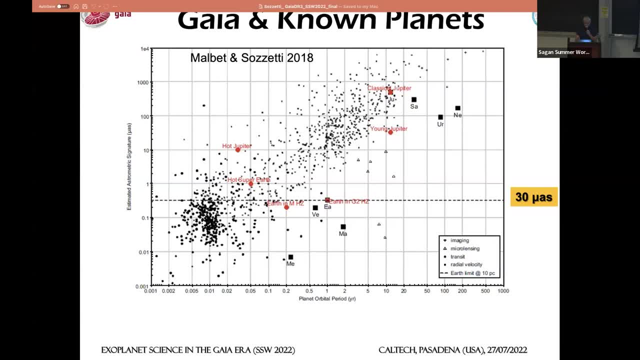 Gaia is said to measure actual masses of these objects And there is an estimate that maybe 50% of the known giant planets from the velocity surveys from the ground are accessible to Gaia for true mass determination And, conversely, we are expecting many Gaia detections. 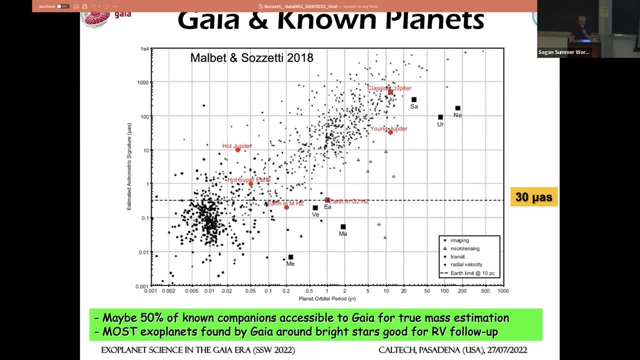 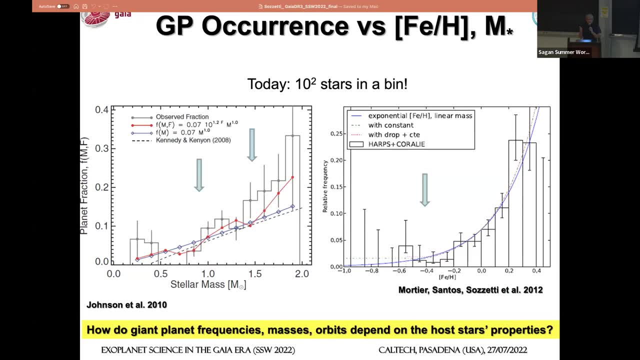 around bright stars, in particular, to be important to start the velocity follow-up work from the ground. When it comes to planetary system demographics, this means looking at planetary properties as an ensemble: occurrence rates and studying them as a function of the properties. 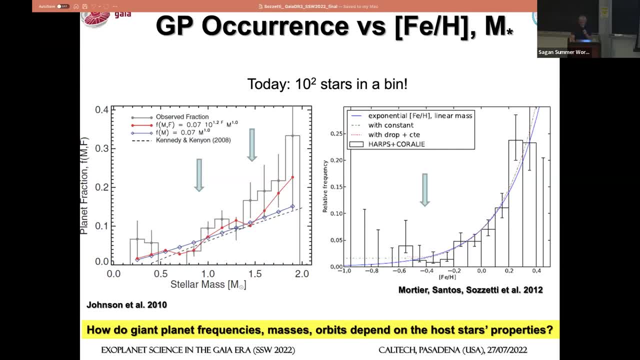 of the planets themselves and the stars they orbit. And these are two cases in which, for example, we know of the existence of clear correlations between giant planet frequency and stellar properties. On the left you see the correlation between giant planet frequency and stellar mass. 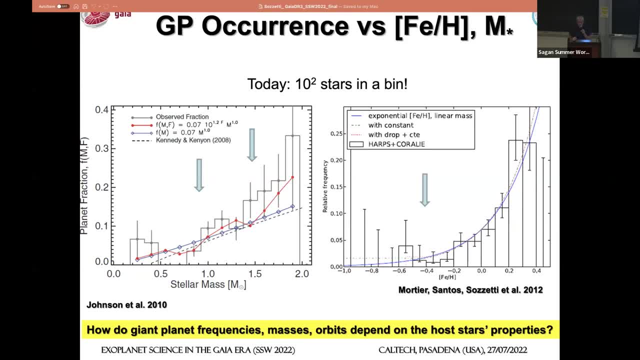 And on the right. instead, you see the rising trend of planetary frequency, with stellar at least visiting chemical composition Today. some of these studies, when it comes to objects with true determined masses, are typically done with these numbers of stars in a beam. 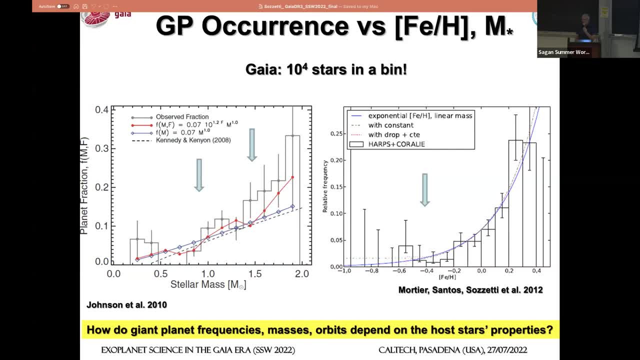 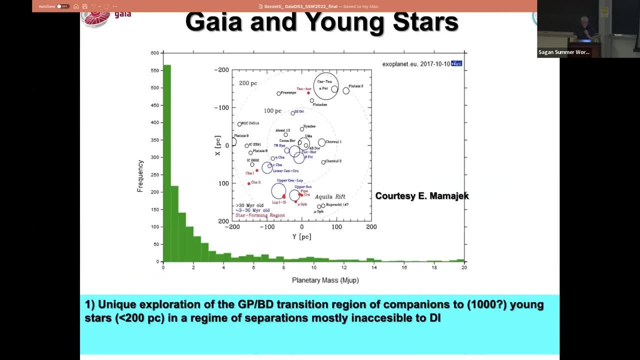 We hope to come up by another two magnitudes in terms of number of stars that can the beams when we're going to be looking at the fine structure of these correlation plots. given the Gaia yield of planets, Gaia will also be accessing stars. 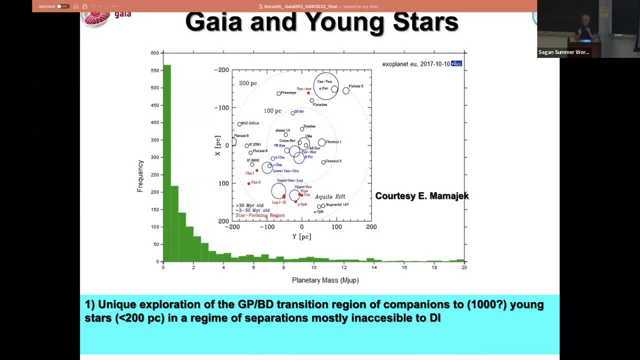 that are very difficult for, for example, for high-velocity work. These are young stars around the nearest moving groups and the nearest star formation regions within 200 parsecs from the sun or so There is a hope to have Gaia be sensitive up to maybe. 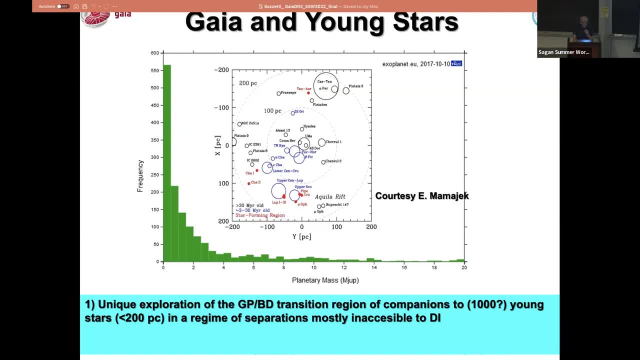 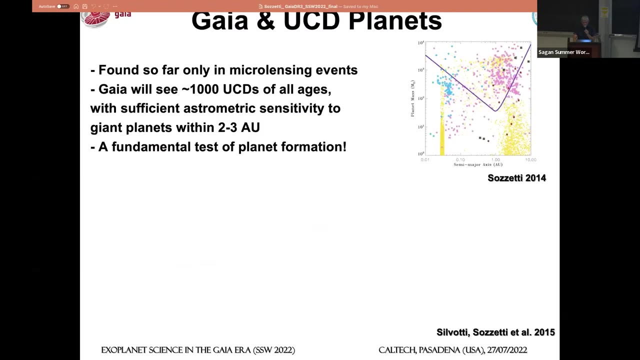 over 1,000 young stars, And this would be a fantastic complement to other techniques that are instead effective. We are funding young planets, but only at very wide separation. This is the direct imaging technique that you heard about a bit earlier on. 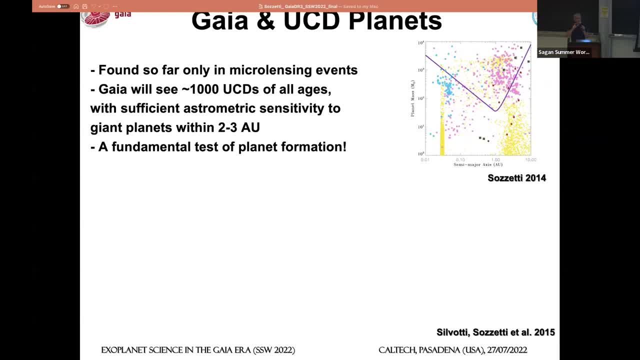 And finally, there are two niches All the way at the extreme ends of star properties and evolution paths. ultra-cool dwarfs are very faint for Gaia, But they're very small and they're found very, very nearby, in the close vicinity. 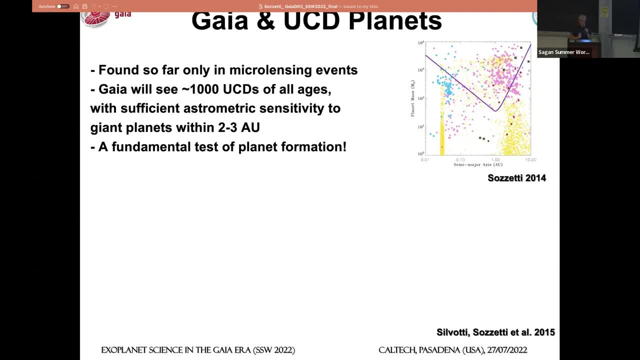 of the sun, And so there is also a forecast that maybe for these hundreds or close to 1,000 ultra-cool dwarfs within 10, 15 parsecs from the sun, that Gaia may actually achieve sufficient sensitivity to also find, if they're there, planetary companions. 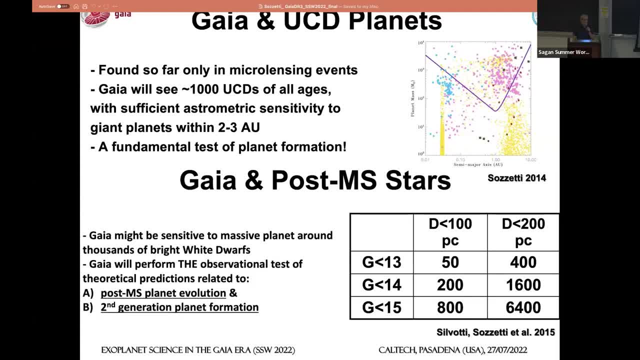 around them And on the other hand, looking at highly evolved stars. the white dwarf population near to the sun is also amenable to planetary detection with Gaia, And here the numbers are potentially of the order again: ballpark 10 to the 3 or so 1,000, already very large. 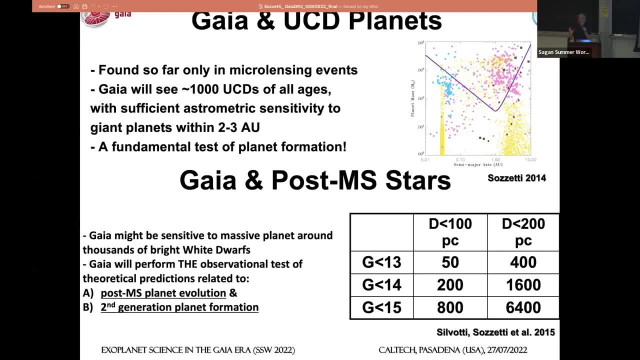 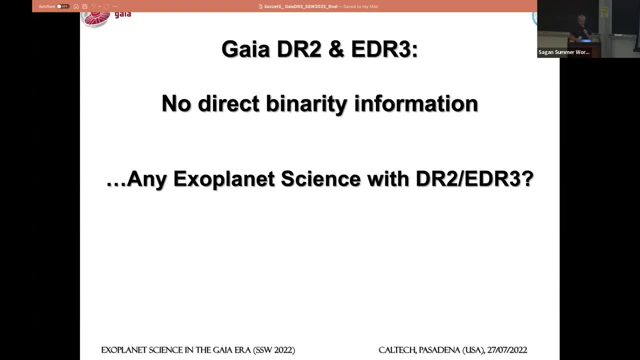 to understand any possible pathways for survival or regeneration of planets around very evolved primaries. Now, a few minutes before we dwell into the DR3 discussion on what has happened today and until today with former data releases. We've heard already this and I will point you again. 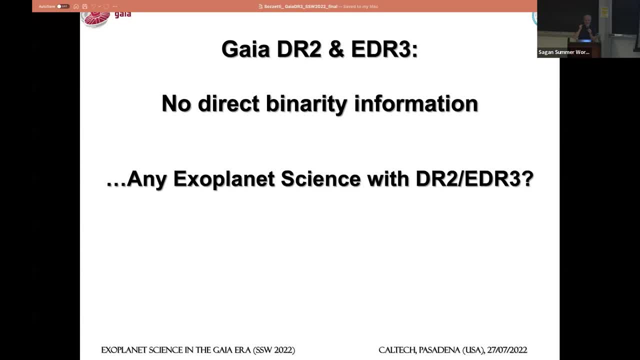 to the talks that have come before me and to the ones that are coming just after me. The key point is that, in principle, there is no direct binary information coming from Gaia: data release 2 and early data release 3.. 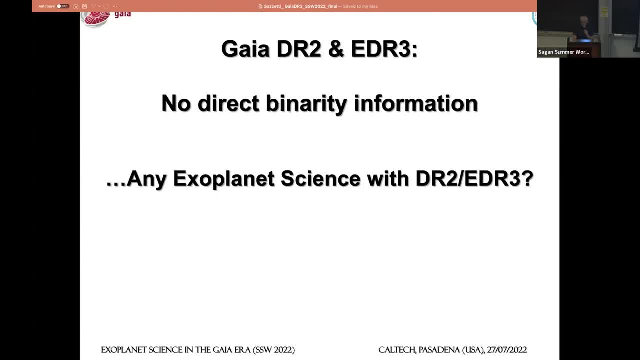 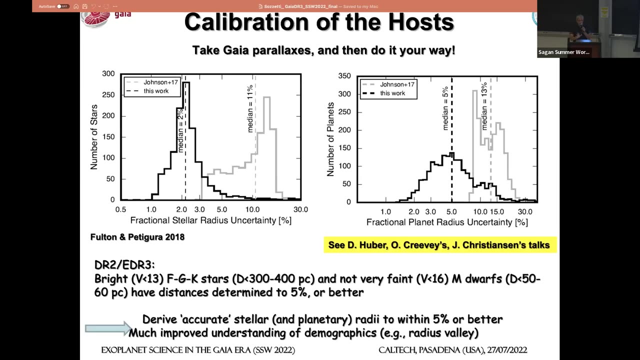 There were only single stars. There are solutions published, But, as we've heard- and I will briefly summarize this again- indeed, exoplanet science has profited from results of Gaia, data release 2 and early data release 3.. The first one was the publication. 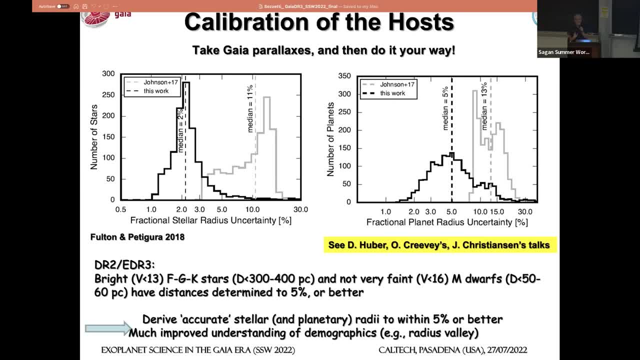 of exquisitely precise direct distance measurements to all the stars that didn't have a parallax measurement before. Those, for example, were the ones in the Kepler field that was observed for detecting transiting planets as small in size as the Earth. 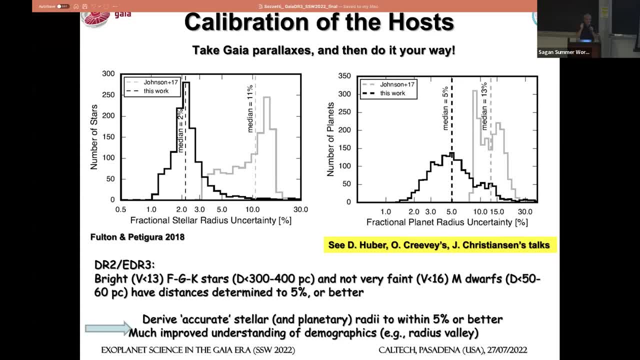 And, in that case, the availability of Gaia parallaxes, as has been discussed by the previous speakers that I'm indicating here, allowed to very much improve the determination of the properties, in particular mass radius, Of the host stars, in turn allowing 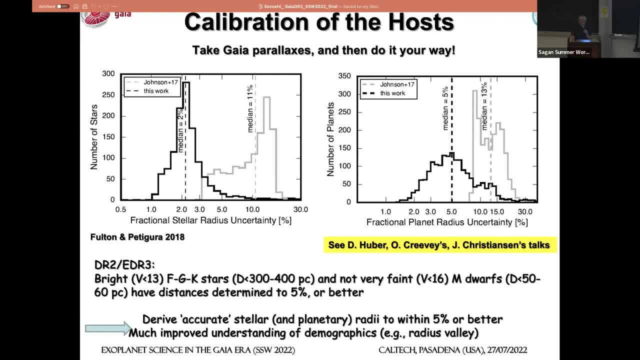 to really determine very accurately the properties of the, in particular the radii, as in this example of the transiting planets, And, as has been discussed by Jesse, this opened the field to much improved analysis in terms of demographics, such as, for example, 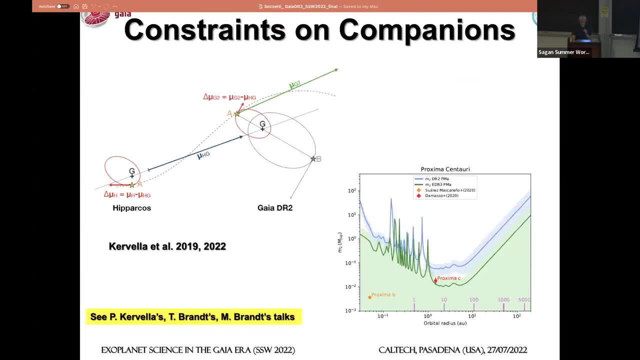 much better understanding of the properties of the radius value. This is for what has come. What's about to come after me I am just briefly touching upon here. There is a very clever technique that was used, based on Gaia data release. 2. 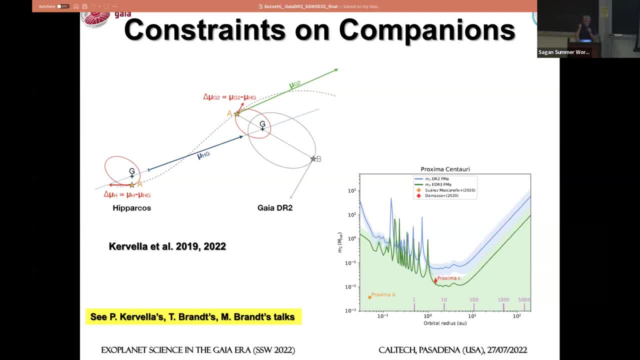 and early data release. 3, where, instead of parallaxes, proper motions from Gaia were used And they were combined were available with Hipparchos proper motions. This combination allows you. I will not get into the details and I will let the speakers after me discuss this. 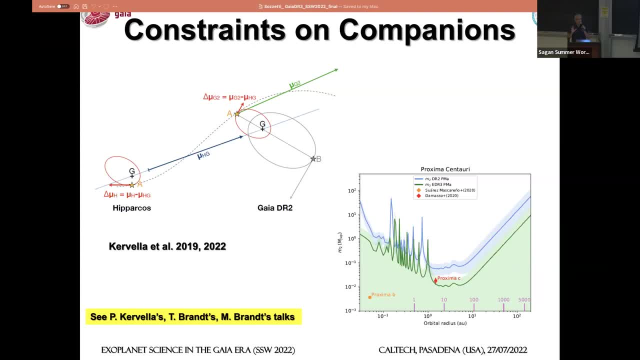 But it allows you to identify variations in the proper motion in the Gaia epoch and Hipparchos epoch that are indicative of the presence of a companion orbiting it. You can do a couple of things with this information. These are actually two points in time only. 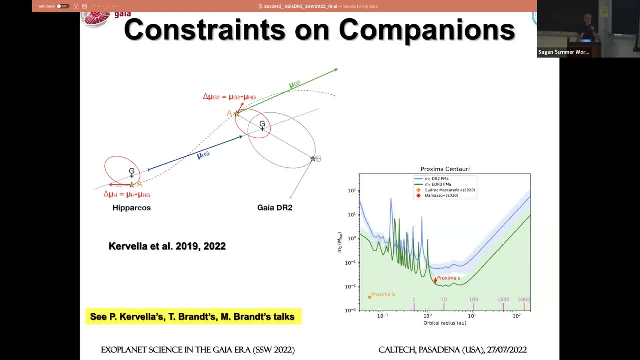 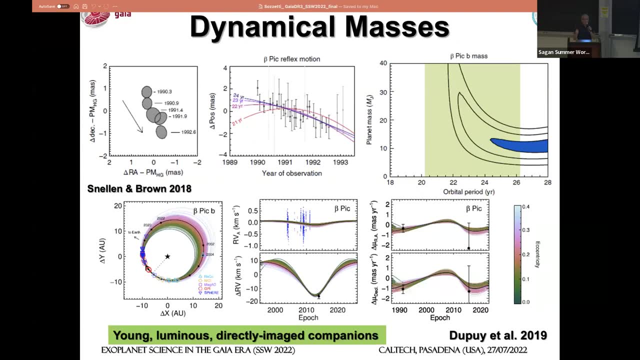 So you cannot really read orbits, But you can place limits, for example, and constraints on the properties of the companion in terms of mass and orbital separation. You can do more if the object is already known to be there, detected, For example. 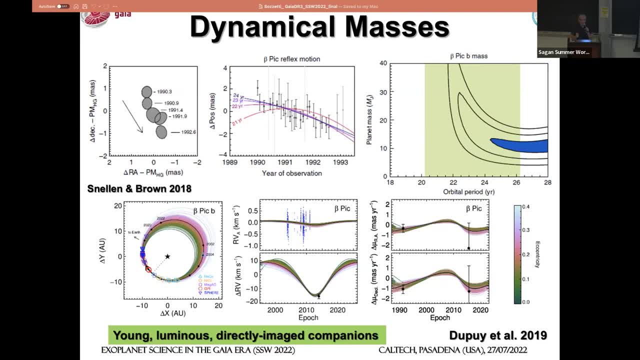 For other techniques. dynamical mass improvements and orbital arrangement improvements can be obtained by combining the proper motion difference technique- proper motion anomaly technique, as it has been dubbed- with other existing data sets such as measurements or direct imaging observations. This is the case, for example, of a very famous high mass. 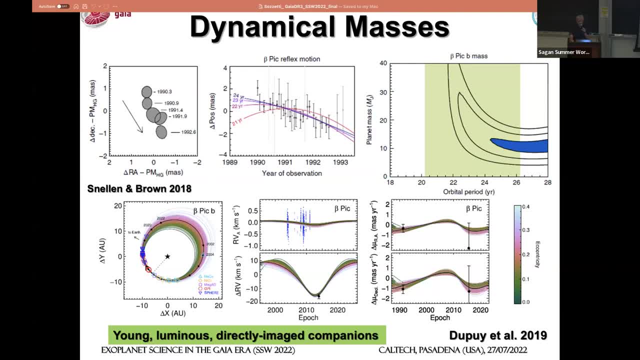 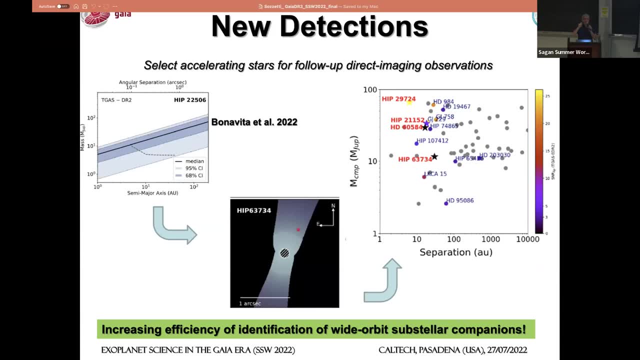 plant, a young high mass plant orbiting the young star Beta pectoris. And you can also do a third thing: You can get stars that have detected acceleration with a proper motion difference that is statistically significant and use them as targets to follow the map and see if you can actually 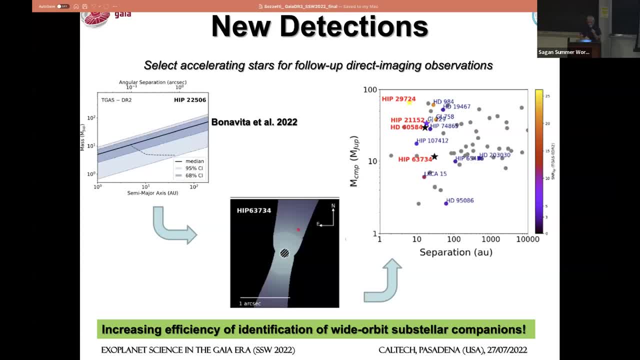 identify the companion. This is, for example, the case of a recent work by Bonavita and collaborators in which in the left you kind of approximately identify the regime of masses and orbital separations that would correspond to the companion. You identify the possible regime of vision angles in the sky. 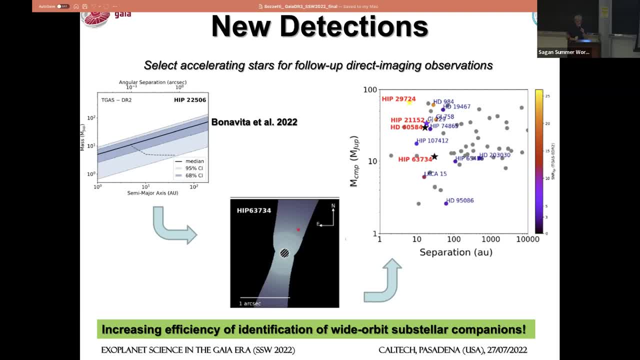 where you could find the planet or the subspecialty companion. if it's there, You indeed find it in the second plot And then you measure its properties and you put it in the mass separation diagram And you increase the efficiency. efficiency and of the detectability of these companions through the direct imaging technique. 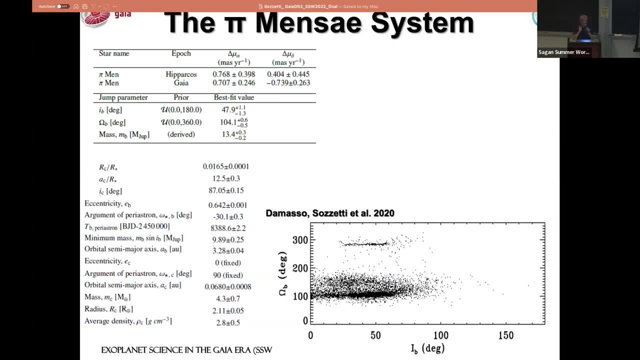 And to conclude, there is also the possibility to more effectively study the details of the specific systems by combining even three different measurements. The PIMENSA system is a particular example of the case in which a radial velocity outer very massive companion on an eccentric orbit detected by analysis. 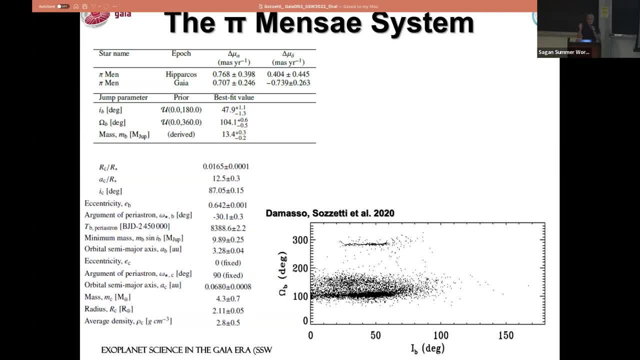 was eventually accompanied in the system by through photometric identification by the test mission by a very close in small mass, low radius super earth and identified in transit. The star is nearby, It's an Ipaco star. It also exhibits a somewhat significant- not super significant, but somewhat significant. 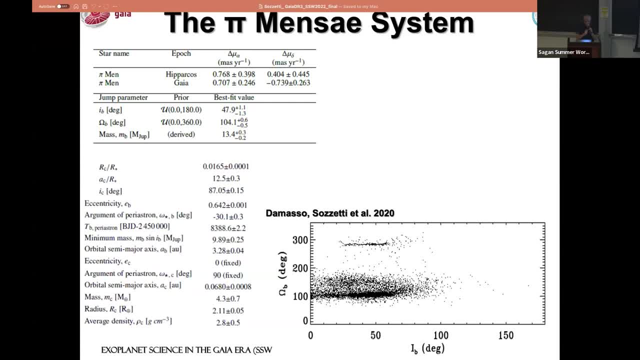 difference in proper motion, as I have discussed before. So you can combine the three techniques and come up with an estimate of the properties of the companion that's producing the proper motion difference. You know there is a transiting companion identified by tests, so you can. 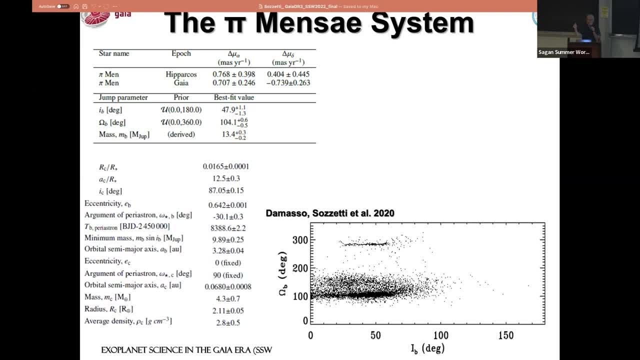 find out, if possible, what is the relative inclination between the orbits of the transiting planet and the outer companion, And you can come up with something that is not, let's say is not, free of degeneracies, because there is an orbital element that is not known by transit work. 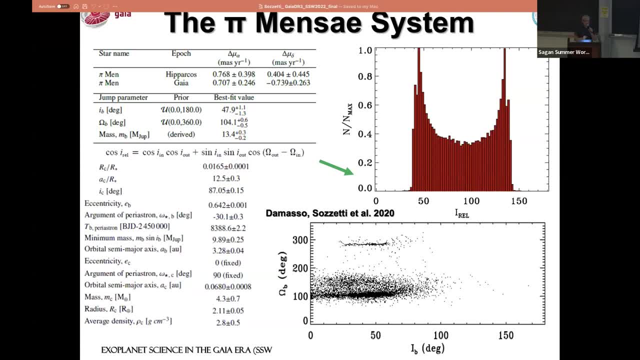 and cannot be determined. This is the longitude of the ascending node, But, however, you can constrain the regime of relative inclinations between the two companions to be at least of order of 50 degrees, And this is one of the most important results that has been obtained so far. 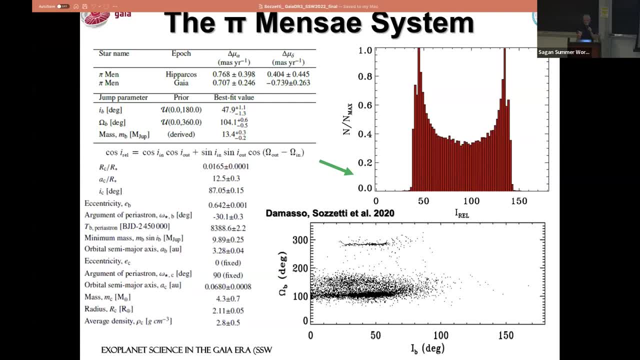 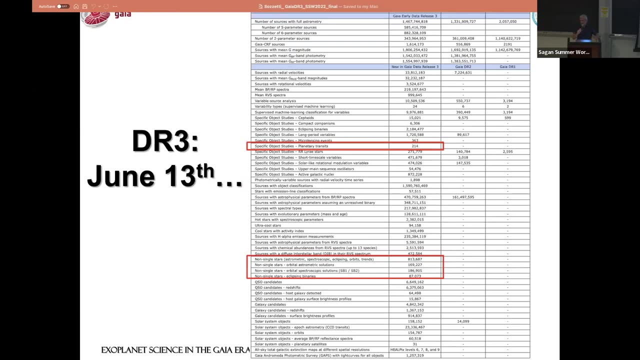 with this, with this combination of techniques, because it is particularly informative for the early history of formation and eventual evolution of the system. Now time to change gears. The second part of the talk and the bulk of my presentation will focus on Gaia D'Astra. 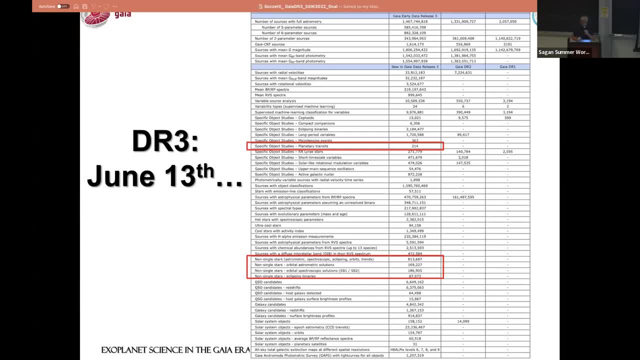 Which has just come out. This is a messy table. I have tried to identify- very hard to read really- the key contributions of Gaia D'Astra to objects identified orbiting other stars. They come in several fashions. There is a class of 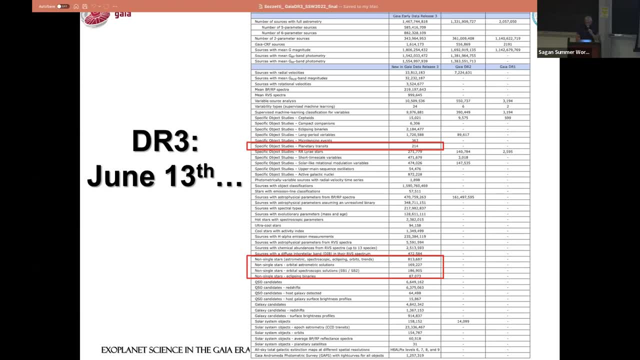 planetary transiting candidates identified there- about 200.. The bulk of it is seen in these lines over there. The non-single star sample accounts for more than 1 million solutions corresponding to the presence of an orbiting companion. This is an outstandingly large number and indeed actually rather modest. 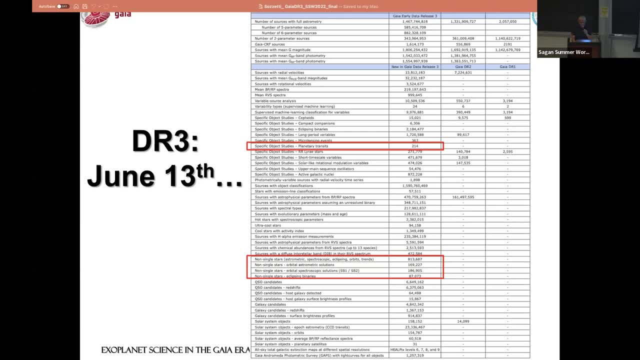 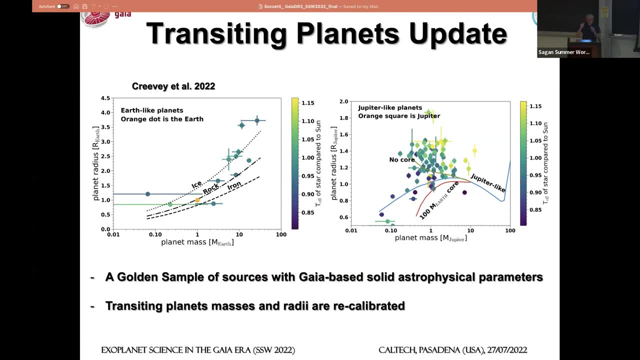 if we think of what's going to happen the next time around, With these results coming out. for DR3,, for example, the group led by Orlok has revisited the issue of the determination of planetary host properties and planetary parameters, improvements solely based on Gaia data themselves. 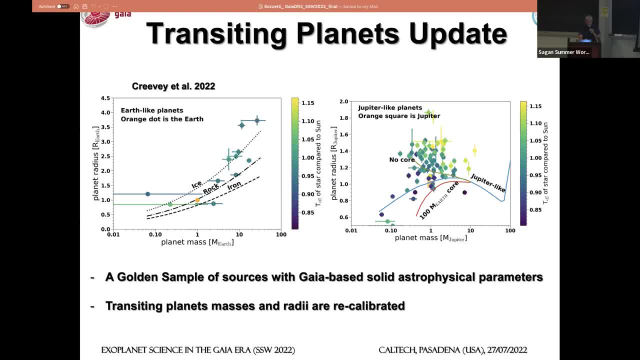 There was an important paper that has contributed to the identification of sources for which Gaia produces a full set of statistical parameters, including masses and radii, that are very accurate And with these you can revisit again the the issue of determining planetary radius and planetary mass. In the left and right panels you see the mass radius diagram for very low. 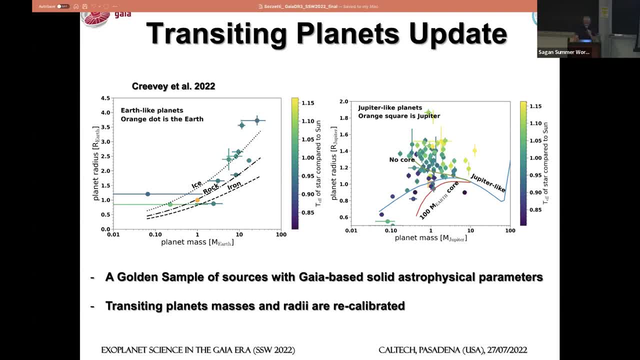 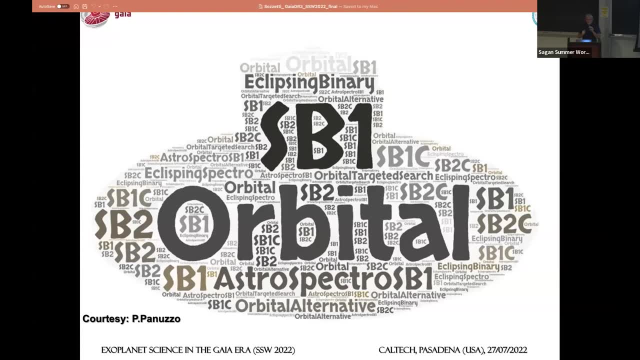 mass, small radius objects and on the right instead for giant planets. this is already being shown by Orlok earlier. Coming to orbital solutions, it's a fantastic dataset, as I said, which is also available on our site. Well, that was a whole big video for you. 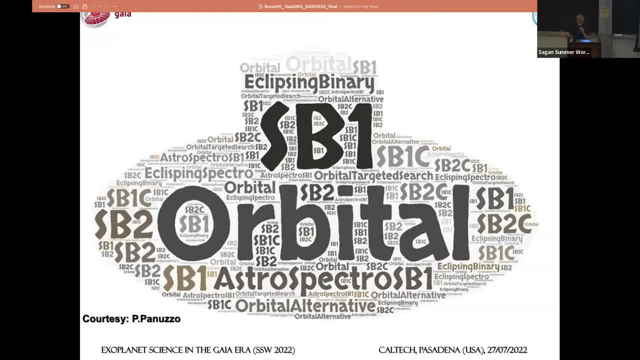 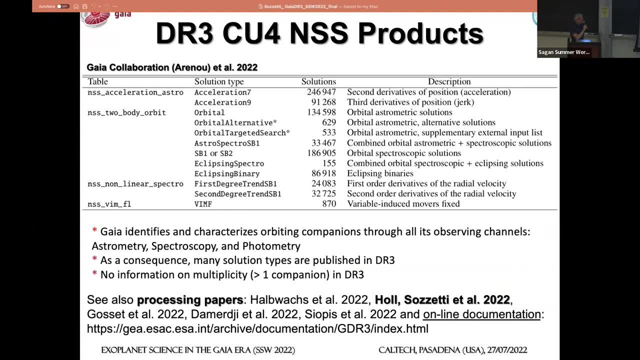 Thank you for watching. See you next time. bye, already said. albeit small, relatively speaking, It comes in a very wide range of flavors because of the different typology of data sets that are used by Gaia to detect them. Companions can be characterized, identified and characterized through all the Gaia observing. 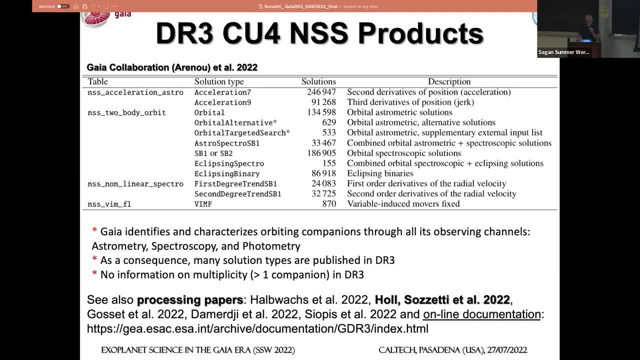 channels- spectroscopy, photometry and astrometry- And, as a consequence, you have a variety of solution types. I will not discuss each and every one of them. I'm open to questions later on. I definitely underline the papers that you see at the bottom of the slide as reference works. 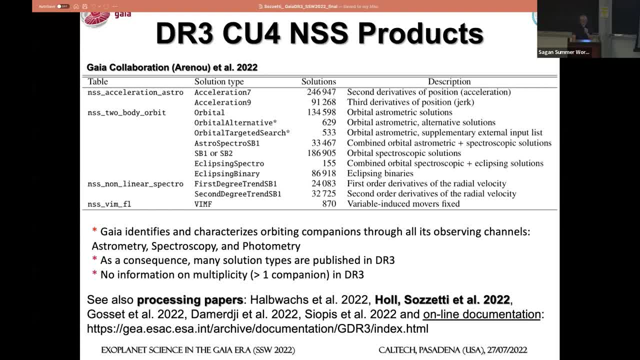 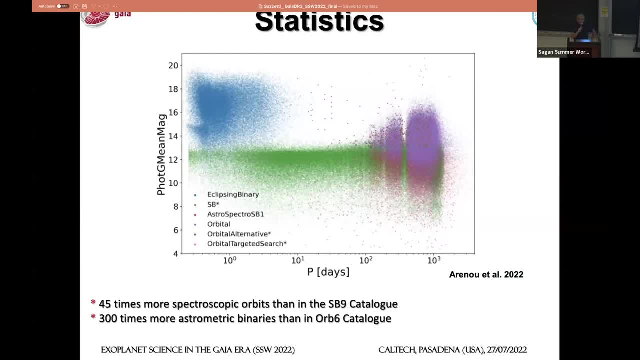 to get very much into the detail of what has been published in the Gaia Archive for the R3 and non-single-star solutions, A bit of statistics. The numbers are already astounding If you take a look, for example, at the comparison between the numbers of spectroscopic orbits. 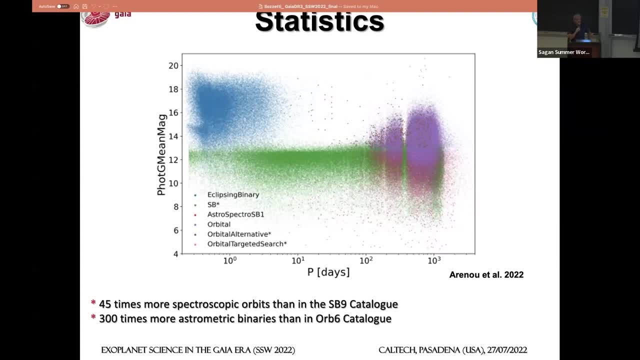 published by Gaia DR3 with respect to the famous SP9 catalog. well, there's only a factor of 45 improvements With respect to existing astrometric binary solutions in the Orbit 6 catalog. we are doing better than a factor of 300.. That's not too bad. You see here the parameter space and 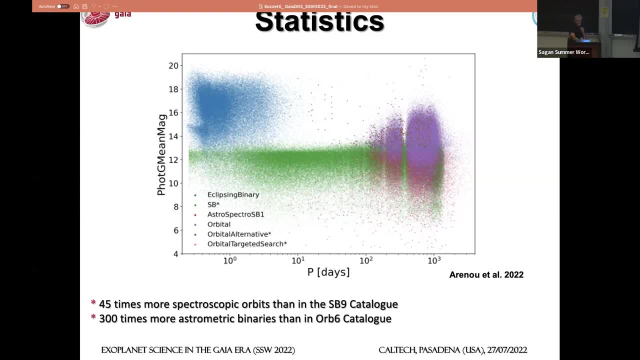 for example in terms of order period covered by the different techniques, And you also see here the clear biases that are intrinsic to the techniques themselves. for example, transiting, eclipsing binaries and transiting planets are only found at very short periods, typically around faint stars, while spectroscopic binaries and astrometric binaries share. 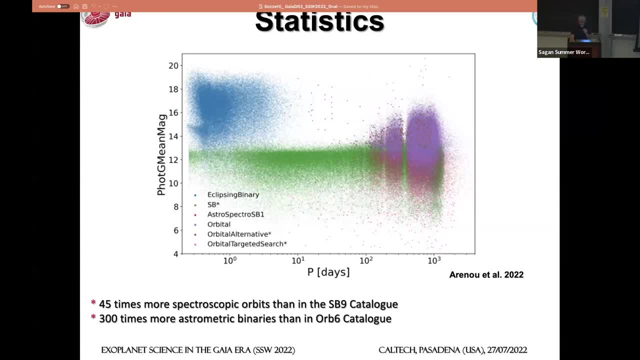 a common region of overlap in terms of sensitivity at periods of exceeding 100 days or so. So this is a very interesting analysis And I hope you can take a look at the data and see how it works. Thank you, I hope you have a great day. Bye-bye. 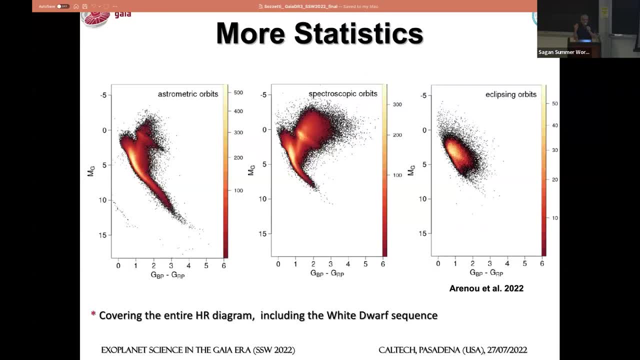 The numbers are fantastic and they allow us to identify companions, essentially orbiting stars, all across the age of anger, particularly with astrometry, but also with social and, to some extent, with eclipsing binary systems. Now there are some excellent news. 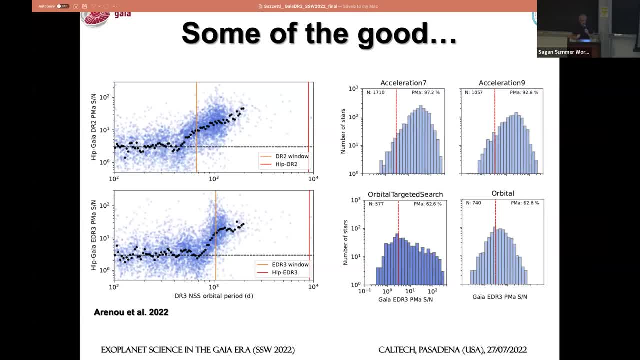 some less so good news. I will touch upon briefly some aspects that are good and some aspects are bad. One element of good news is the fact that we were expecting to identify and to correlate the presence of an orbital solution in Gaia-DR3 with the fact that the star may have. 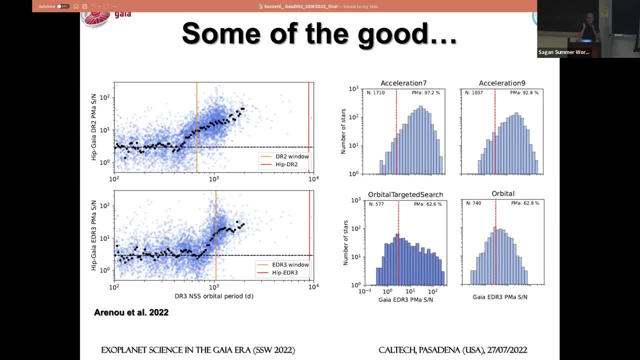 already been known to have an acceleration through the Gaia-Hiparcos proper motion technique. In the diagrams on the left you see indeed that when the signal-to-noise ratio of the Hipparcos-Gaia proper motion difference increases to a negative degree, the power of air or air-to-air 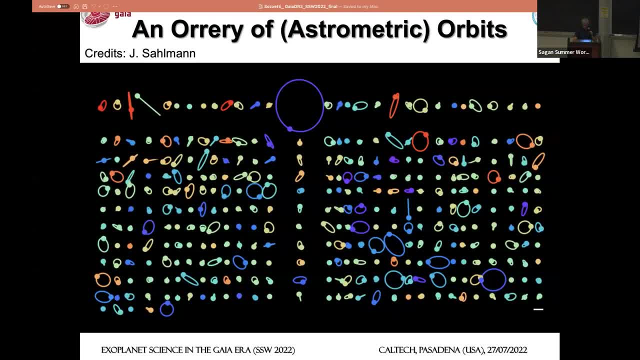 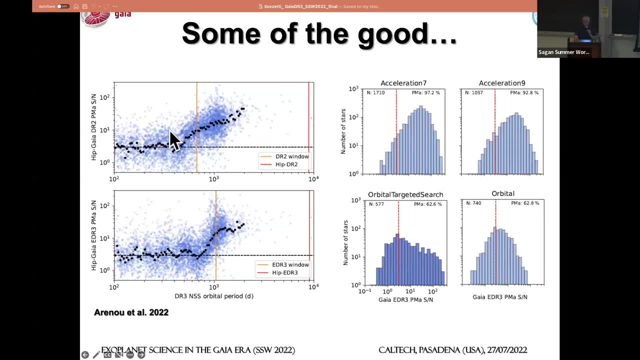 is very high. yeah, i have to do it like this. yes, here, when the high signal noise ratio, when the signal noise ratio of the propulsion difference is high, you begin to see a clear correlation with the period of the orbital solution or the defining idea. this is good news. 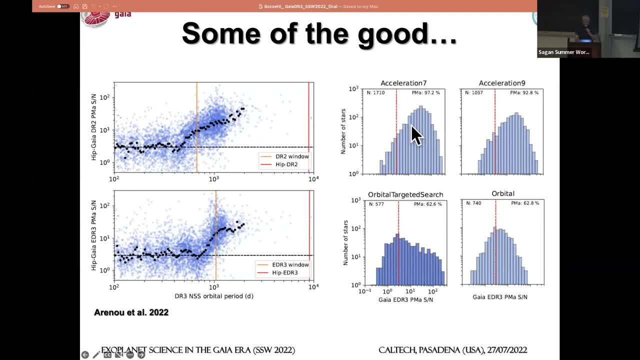 because we are expecting it's actually happening also for the class of orbital solutions that are the correspond to acceleration solutions described in gaia. in gaia data release 3, they come in two flavors. in successively higher order derivatives of the proper motion, these indicate the presence of a very long period companion whose orbit is not entirely. 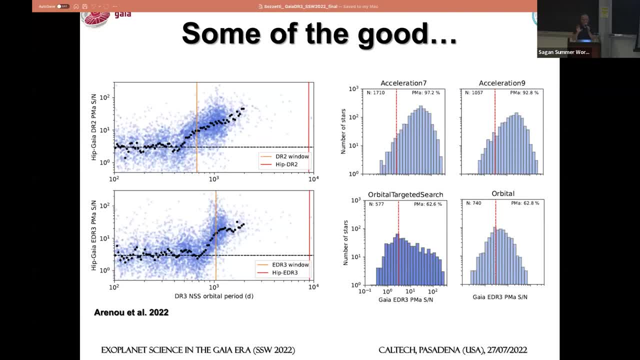 these are expected to be captured by the guy- yeah, promotion anomaly technique, and indeed there is a very high fraction of these that turn out to be found also by the promotion anomaly technique. this is all good news and, conversely, for those for which you have a full orbit, indeed, you do not expect as such a large amount of overlap. 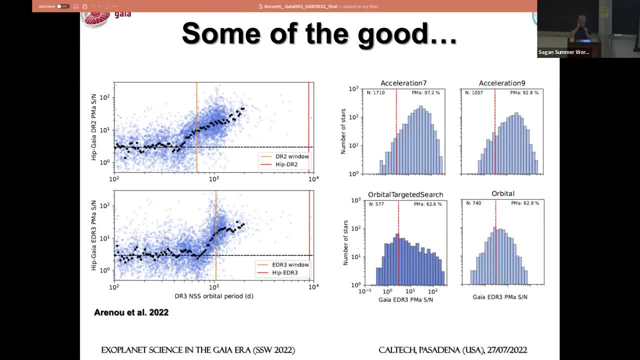 indeed, there is a lower fraction of objects with both promotion anomaly as well as full orbital solution. these could be due to could be interpreted in two ways. uh, possibility number one: there is a long period companion and gaia has fit in an orbit that is significantly underestimating the orbital period, the true orbital period, or guy has found an orbit of. 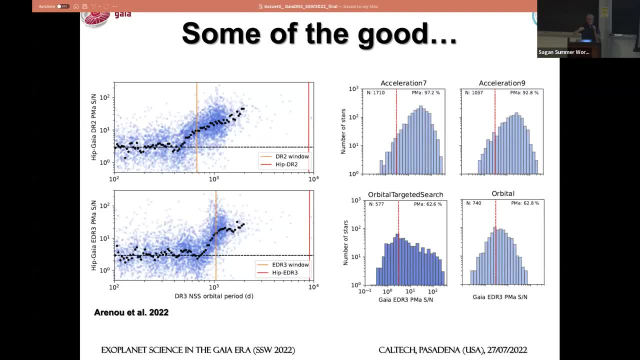 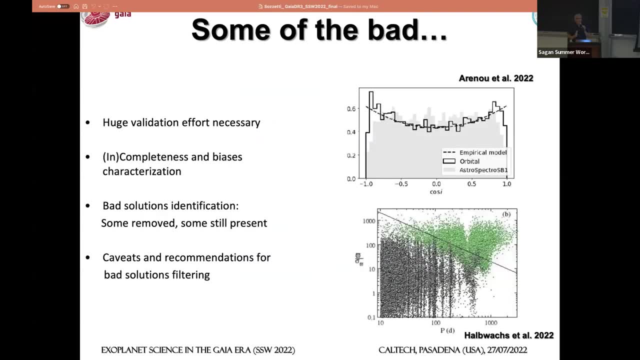 a companion and there is another outer companion and the proper motion anomaly is indicating the presence of a companion that is not the one detected by gaia. these are very good news. there is also some bad news, but we do know that, if the this was to be the case, more than the real objection to the 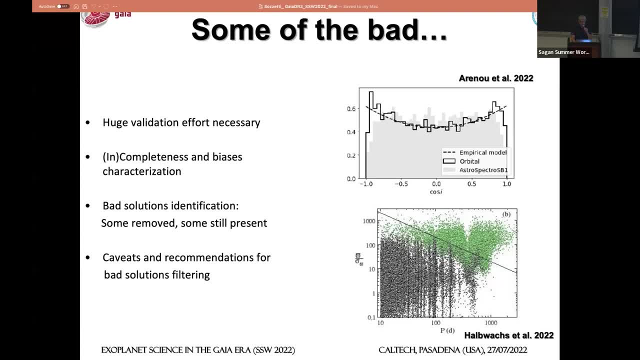 Awayyss produit would be to actually solve our problems the way binaries, so the kind doors on the next slide which viennent from wesleyan, an already justice options gettingway from california has three seen many bad solutions that we had to discard And unfortunately not all of them. 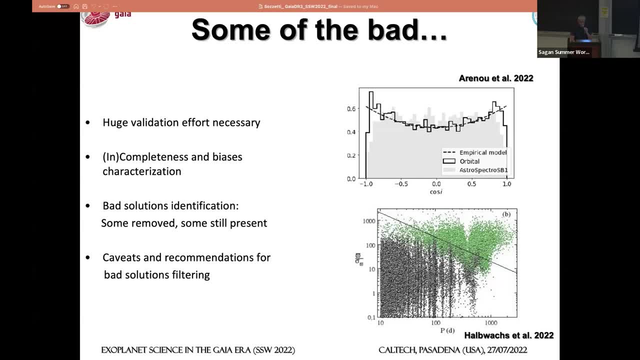 have been able to be vetted entirely, And so there are still some things that are scurrious in the Gaia catalog, And we have done the best we could in order to identify the caveats and provide recommendations in order to handle the data as best as they can. 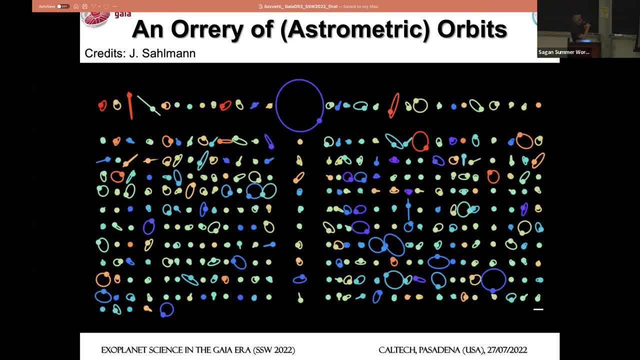 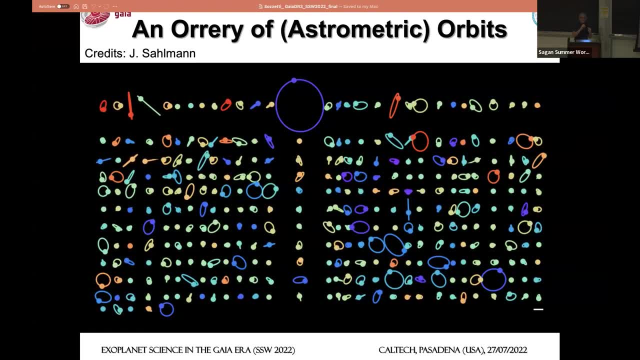 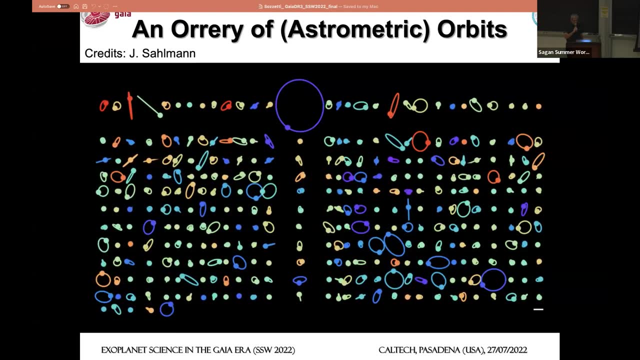 Nevertheless it's spectacular. This is not entirely original. The first version of the orbit already was produced by Dan Fabrici for the Kepler mission, But this applies to full orbits with Gaia's geometry And indeed it still looks spectacular because you see things of all sorts. 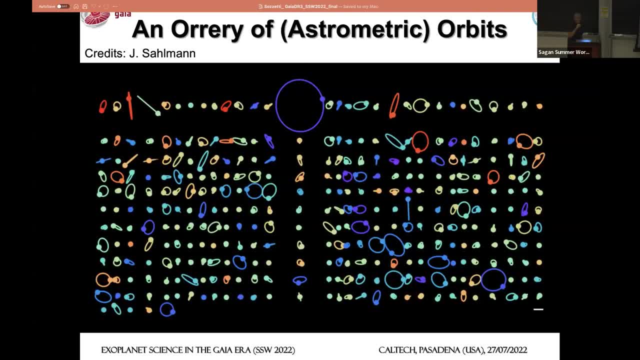 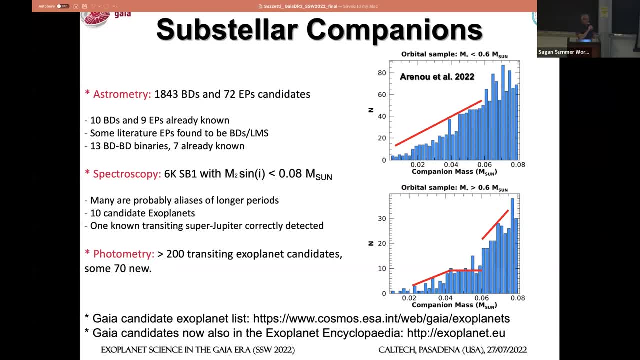 Perfectly round, super eccentric, oriented, all sorts of ways in the plane of the sky. We have to talk about planets and sub-stellar companions, So let's get down to it. We have already heard through Michael's talk, the global numbers. 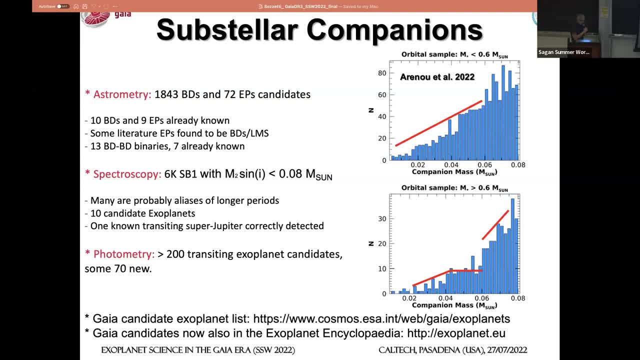 I re-summarized them here. There is approximately an order of 2,000 sub-stellar companions identified by Gaia-DR3 through the various channels. A couple of thousand, sorry, So an order of 2,000.. A couple of thousand through astrometry. 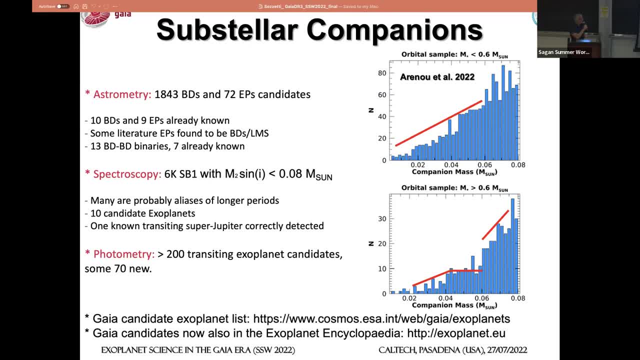 An additional couple of thousand through spectroscopy, An order of a couple of hundred through photometry. You see here the summary of the numbers exploited by the different techniques. Astrometry has contributed particularly in identifying better properties, better orbits and true masses for some of already known. 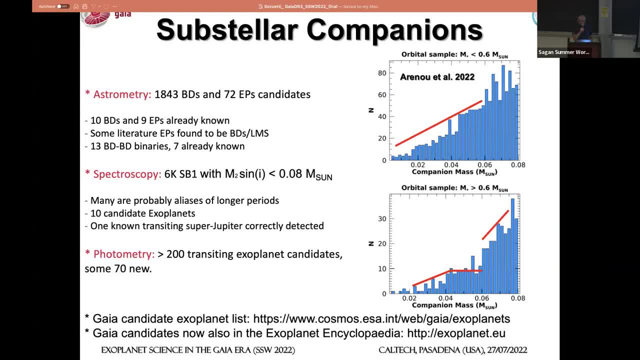 brown dwarfs and exoplanets. It has found some surprises And it has identified objects that were thought to be exoplanets to be, instead of a different nature, Much more massive objects- brown dwarfs or Loma stars- In spectroscopy. right now we are 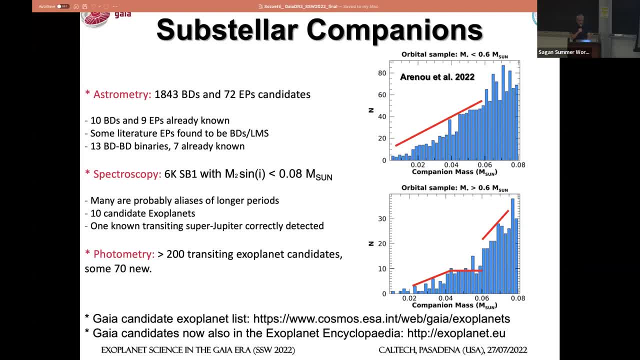 attempting to play it a little bit safer. This large sample of spectroscopic binaries with very, very low mass companions- minimum masses- is potentially populated by a large amount of orbits that are not correct. They are eyelesses, They are short-period orbits, eyeless to a very short period. 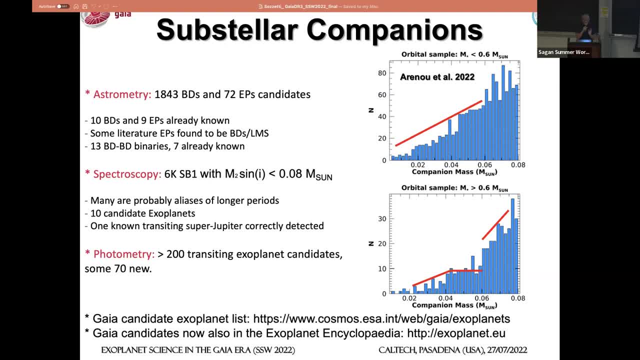 But indeed the companion that is producing the motion is a very long-period object. So right now we are trying to play very safe And we have identified only a very small sample of objects that we can consider robust, And we have identified some very large candidates. 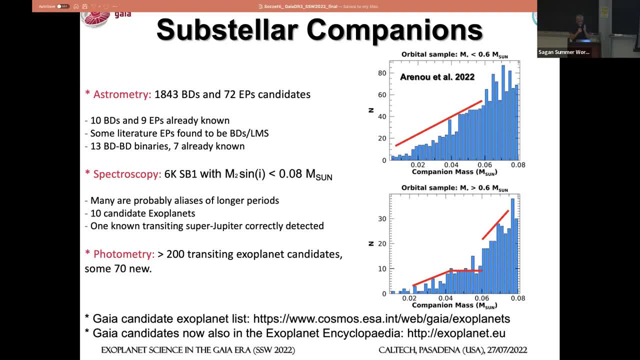 in the exoplanetary regime And for photometry. out of the approximately 200 candidates, there is a majority of objects that were already known and were actually used for validation purposes to verify that the results were indeed performed correctly, But there is over 70 new candidates. 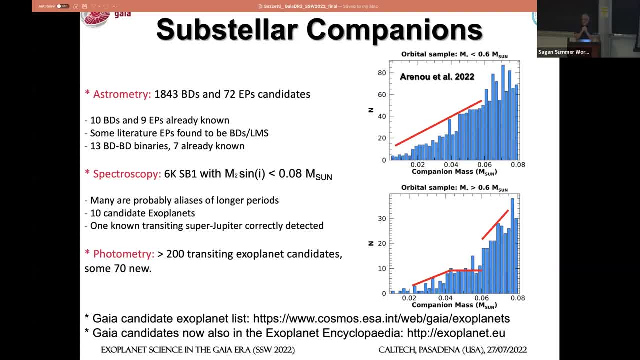 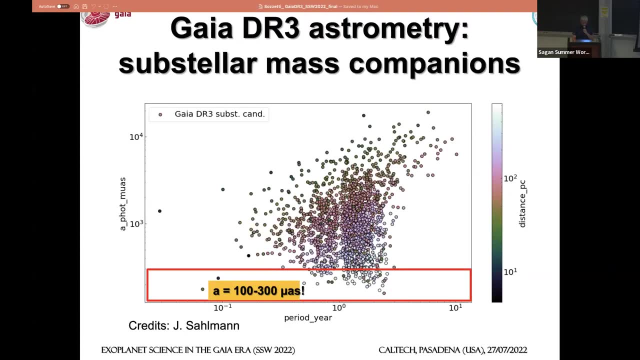 The full list through the three techniques that you see here and is going to be routinely updated on the GEI website, And there is also now an equivalent that has been captured just a couple of days ago and is available through the Exoplanets Encyclopedia. 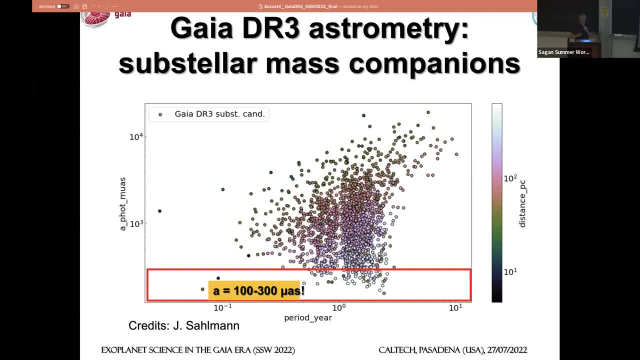 The three astrometry will be the bulk of the rest of my presentation. I first of all want to highlight the fact that, when it comes to orbit size that has been detected by GEI Already at the level of GEI-DR3, we 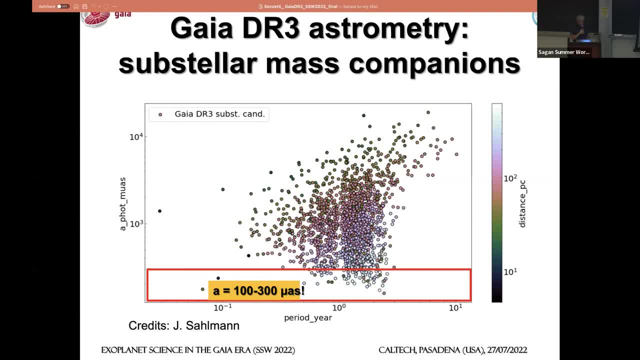 are going down at the bottom of this plot that I show here in the order of a couple of hundred micro-second regime. These are already sizes of somatic perturbations that are really small And with these numbers we are beginning to really touch upon the population of perturbations. 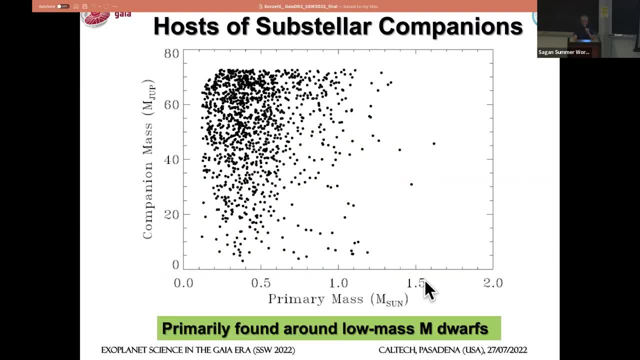 that are produced by planets. We were expecting- and indeed this is the case- that, with the limitations of GEI-DR3 that I will touch upon at the end as a summary, the vast majority of the objects for which we had the chance to identify. 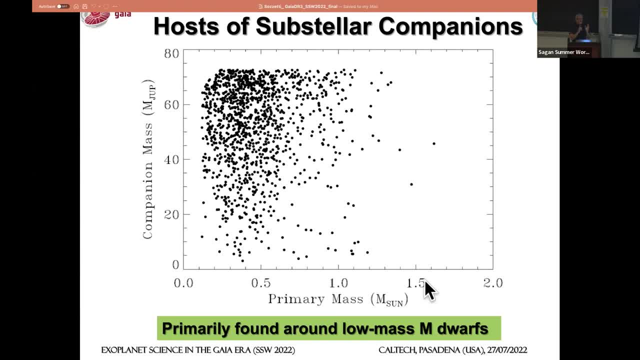 an orbiting companion in the substellar regime would be the lowest-mass stars. And indeed in this plot you see the bulk of substellar companions, their masses as a function of the mass of the primary, And you see the overwhelming majority. 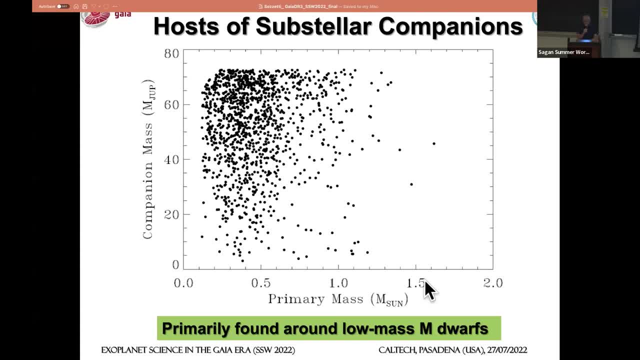 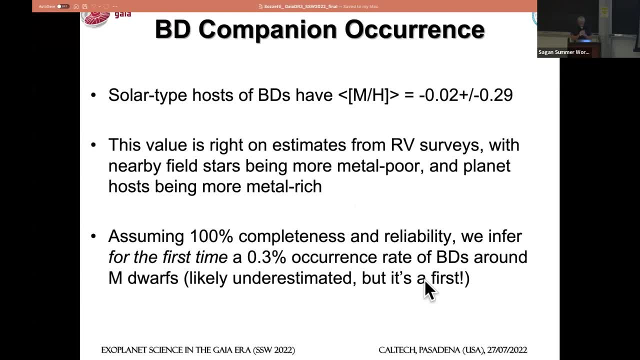 of objects identified by GEI-DR3 through astrometry is orbiting stars with half a solar mass or less. This was entirely expected. We can begin and now remember the slides that I provided at the beginning as examples of what GEI-DR3 can. 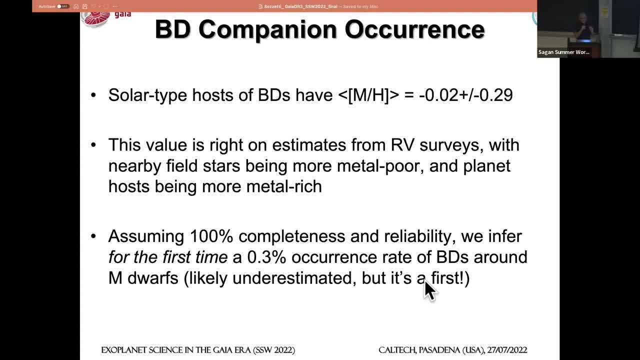 do, We can begin to do statistics, not with the planetary sample that you have seen- It's still rather small- but certainly with a brown dwarf sample of objects identified. Now we had a checkpoint that we were happy to identify as correct. 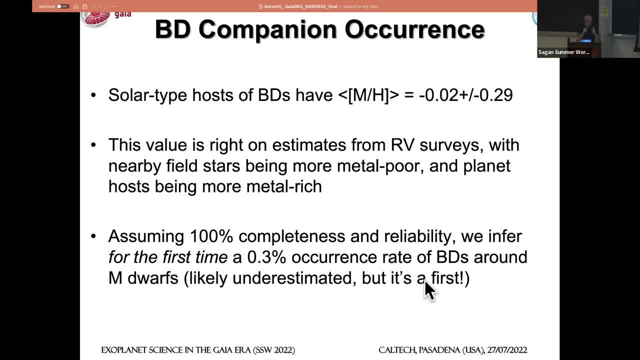 The hosts of brown dwarfs. this is a relatively small number. when it comes to solar-type stars, as you have seen for the previous plot, have chemical composition that is essentially identical to the sun. as estimated to, This is a number that matches exactly the inference. 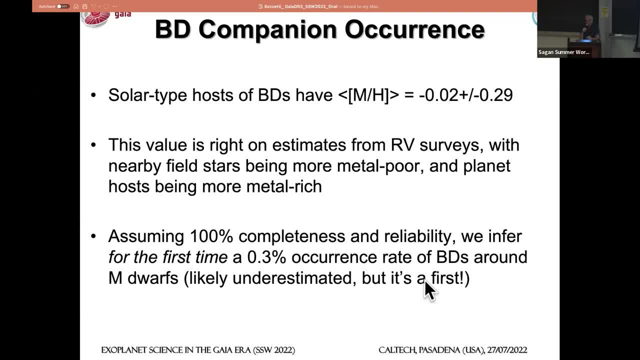 from rather velocity work that has identified solar-type stars with essentially this distribution that is exactly solar, And this is reassuring that we are doing things right, because it is known that in the field, stars not known to host planets or brown dwarfs are a little bit metal poor in the neighborhood of the sun. 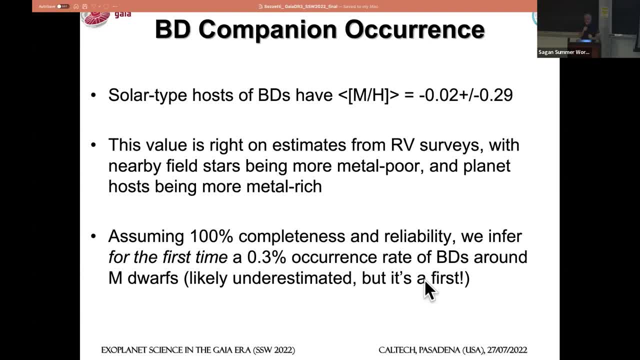 And the planet hosts instead are definitely metal rich, And so brown dwarf hosts fall approximately in the middle. Another thing: you can do with a much larger sample of brown dwarfs that has been identified around the lower-mass companions, the M dwarfs. assuming everything is fine, 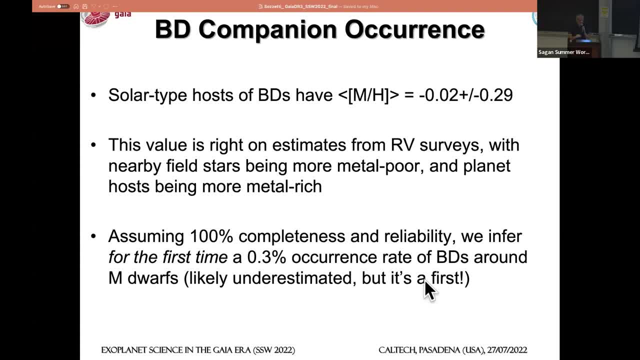 that we are perfectly complete and fully reliable, which is certainly not the case. you can make a first inference on the occurrence rate of such companions around low-mass stars, And this is the first time that such a number has been produced. We are expecting this to be an underestimate. 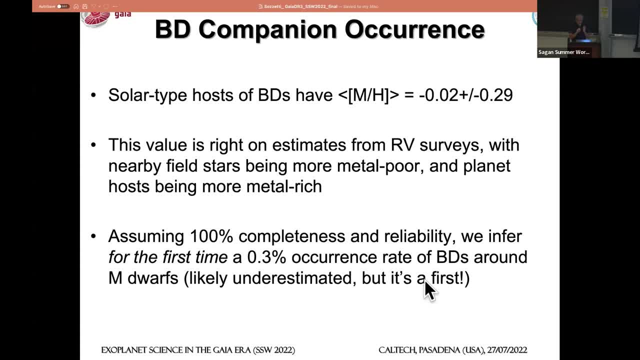 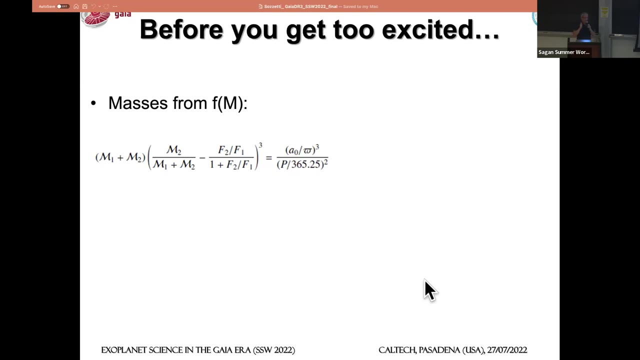 because certainly the survey that has produced the DL3 archive is neither complete nor fully reliable. So we are missing objects And we certainly will see this number rising, But it is a first timer in any case. Now let's get instead to something that is not so good. 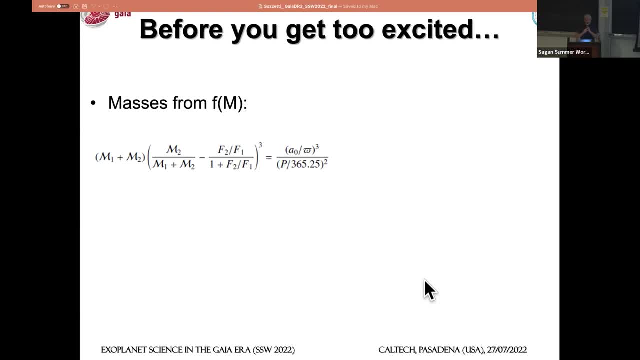 And these were all excellent news For astrometry- you can determine the so-called astrometric mass function. This is the equation that you see here. You have on the right side the size of the perturbation, the parallax, the orbital period, and on the left 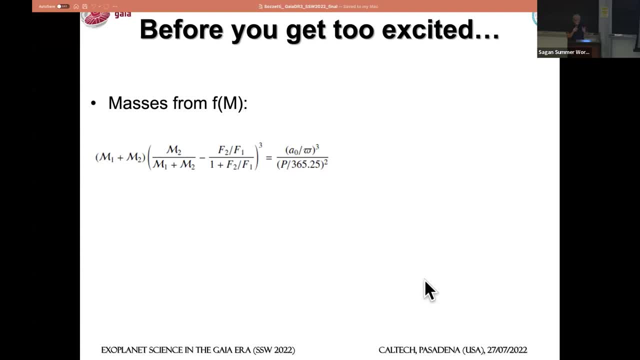 a combination of the mass ratio of the companions, the primary and the secondary, and the flux ratio of the object. The first thing that I would like to point this to you is that be warned that this is going to come back if you choose to go through this challenge. 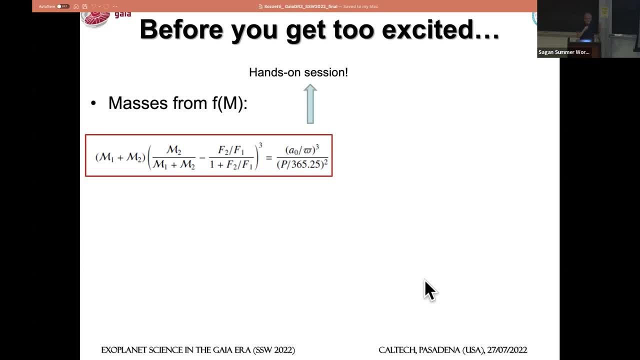 of the hands-on session fitting Gaia-like observations to try to determine the orbit and the mass of a companion. We'll go through this equation in order to determine its true mass once we have found its orbit. So keep it in mind and write it down. 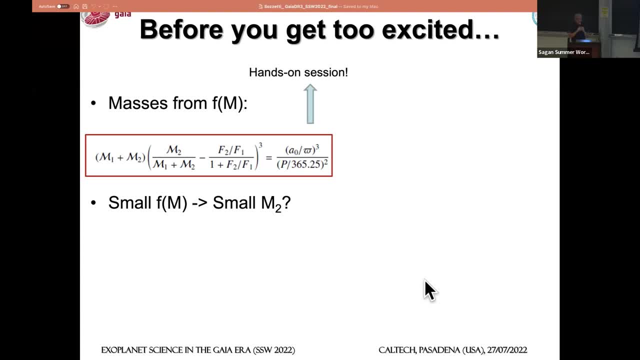 Now here's a question for you. If I have a small value of the mass function, does that mean that the companion has a small mass? How many of you think this is the case? Raise your hands. Nobody. If none of you thinks this is the case. 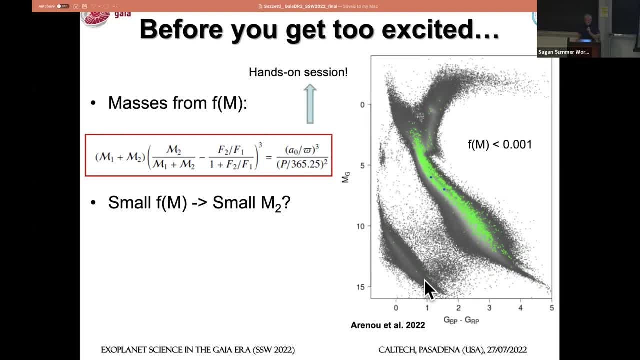 then you are really right, because, indeed, if you have a very small mass function, you still have an ambiguity, And you see this perfectly displayed in the column monitor diagram. on the right, The green dots are the objects for which we have a very small mass function, less than 10 to the minus 3. 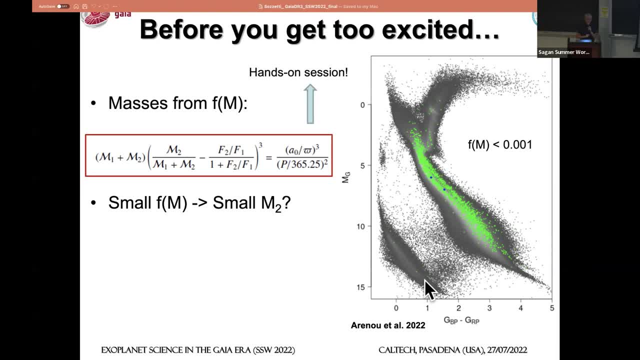 in the Gaia-3 archive with an orbit solution And you see on the HR diagram a clear splitting of the main sequence And you see the same thing here. This is not very good news, in the sense that you are identifying objects that are clearly over-luminous. 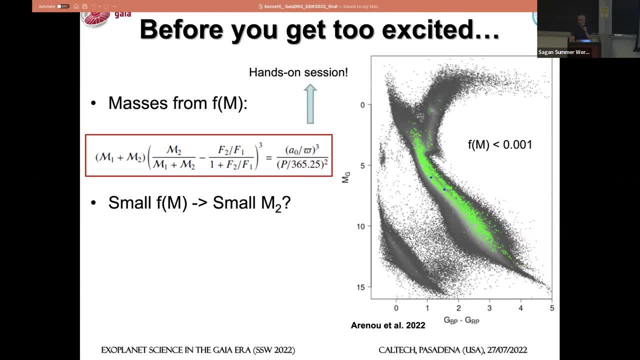 And so the companion that you are seeing, indeed, is not an object that is orbiting a star with a small mass, but is indeed an impostor. This is a class of systems for which the mass ratio is almost equal to the flux ratio. 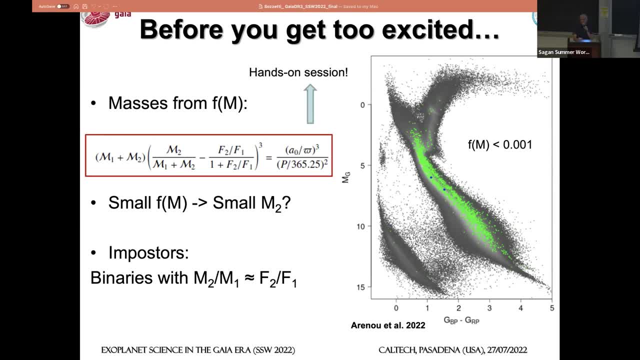 And, as a consequence, you get a very small mass function. You get a smaller mass function not because the companion mass is small, And there's a significant population of these in Gaia-3 that we have been able to catch directly, essentially just. 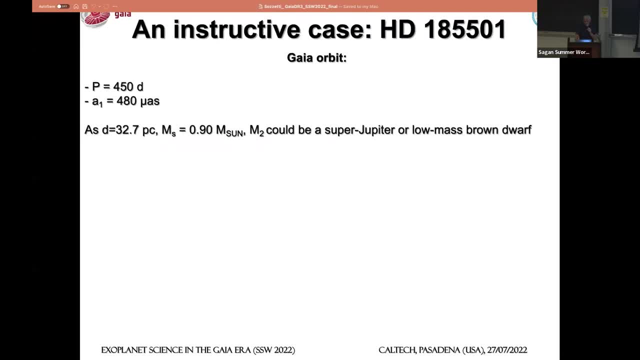 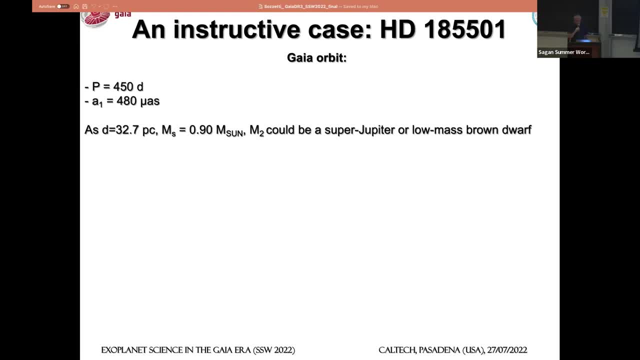 This is a nearby star of 3,3 passex or so. Assume a solar mass approximate for the primary, you come up with an inferred mass of the companion in the low mass-perm. draw for very super Jupiter kind of system. Indeed, there is a published orbital solution. 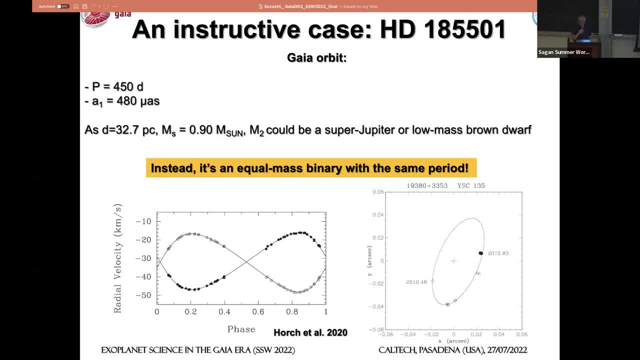 to speckle astrometry and velocity back two years ago. that says it's an equal mass binary with exactly the same period as detected by Gaia. So this is a clear example of the type of impostors that are certainly lurking in the data. 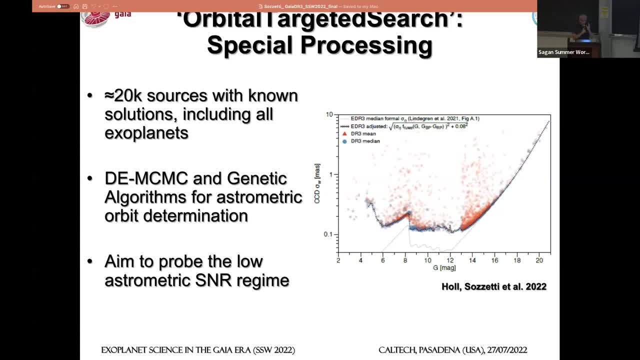 To reach towards the end of my talk, I will now focus briefly on a specific aspect of the analysis and the processing that has been carried out, specifically to try to dig up astromagnetic signals due to very low mass companions in the regime of very low signal. 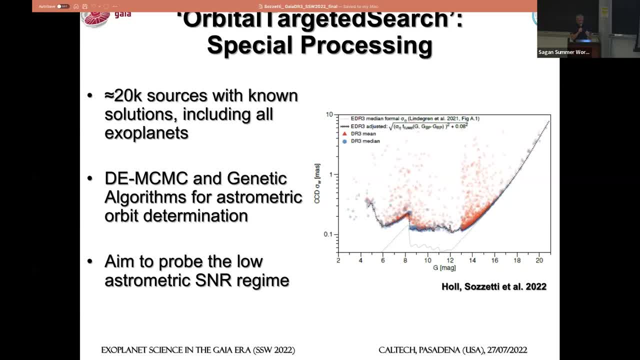 to noise in the astrometry. This is a work that is specifically focused on a selected sample of approximately 20,000 sources with known orbital solutions, including all the known planets, brown dwarfs, astrometric spectroscopic binaries. We tackle the problem through somewhat. 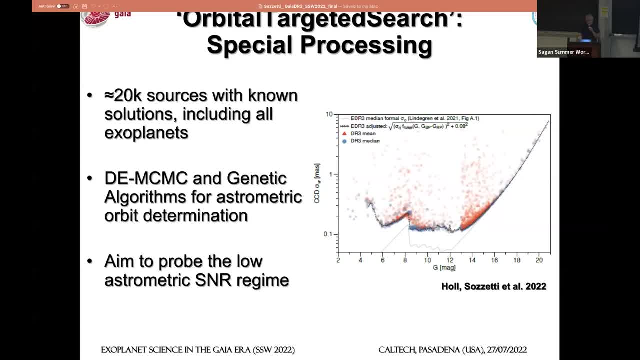 sophisticated orbit fitting techniques. I will not get into the details here, but I will now tell you a little bit more of how things are done in the next slide. And we have to deal with many difficulties. One difficulty you see here, for example, in the plot on the right: 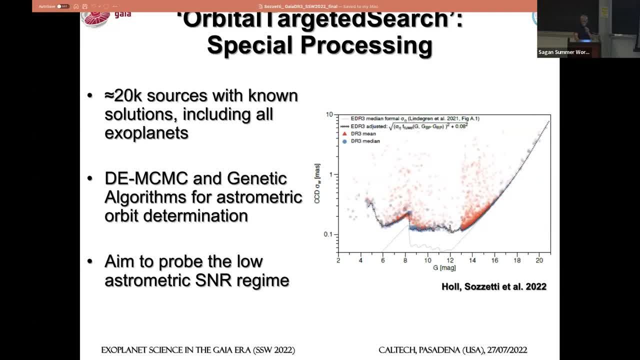 the median error in the Gaia astrometry at the CCD level is the big curve of the values. This is the median, This is the mean of the values. You see, there are many, many data points that we had to use that have, let's say, suboptimal uncertainties. 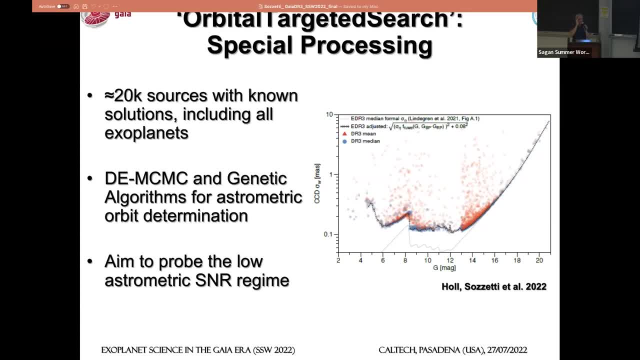 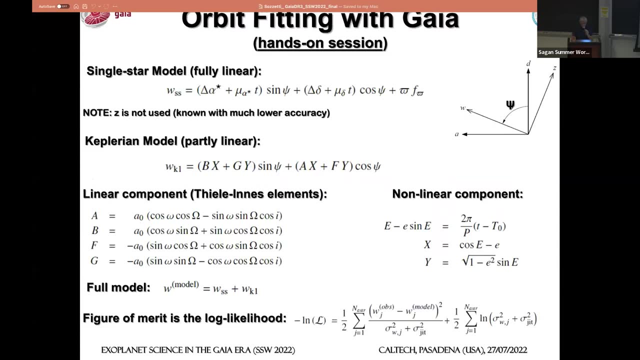 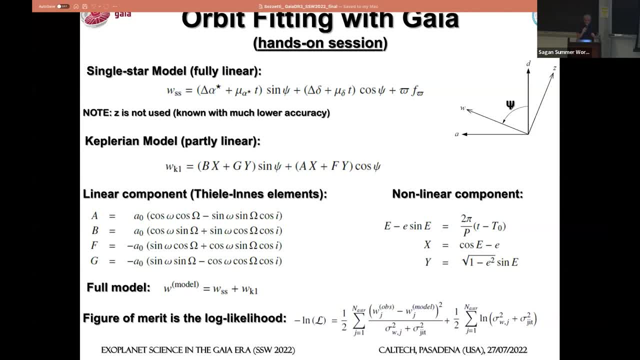 of all the ingredients that we use for orbit fitting, We apply the combination of a single-star model, five astroventric parameters for motion parallax positions rotated along the scanning direction of Gaia. So we use only- as it has been already underlined- 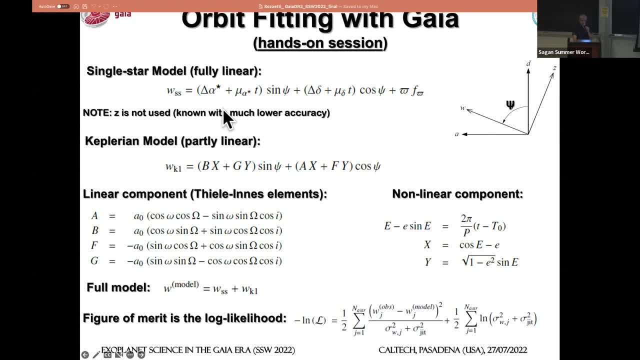 intrinsically one-dimensional observations. We don't use the other direction, what we call the coordinate z, which has much lower accuracy. We model the five astroventric parameters combined with an orbital model that is described here. This is again the rotation along the scanning direction. 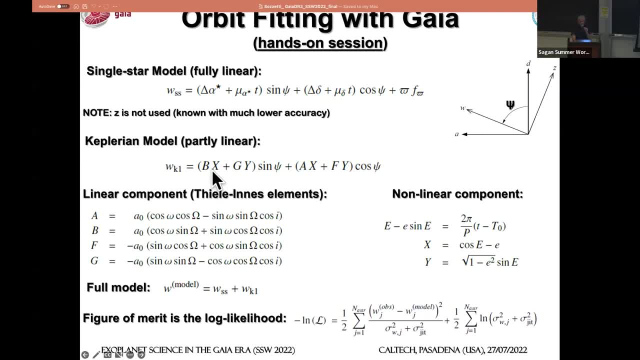 of Gaia. This is the orbital effect, which is the combination of these two terms. The parameters a, b, f, g are what we call the Tillings elements. They are a combination of orbital parameters that allow to make the model partly linear. 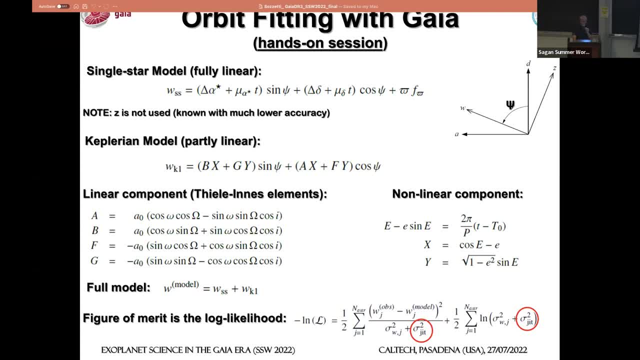 There is an unavoidably nonlinear component of the model that captures the three remaining orbital parameters: the time of periastral passage, the orbital period And the eccentricity- And you will see, if you go through the exercise of orbit fitting that you will have indeed. 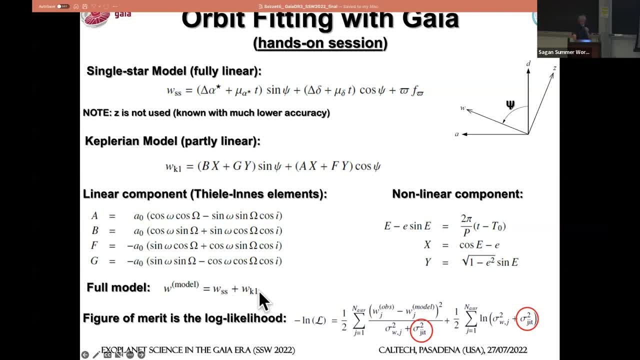 to deal with all these equations. The full model is a combination of the two, as I said, And then we chose, given the specific type of Bayesian approach, a figure of Manet. that is the log likelihood In this. you see here something that, in case you, 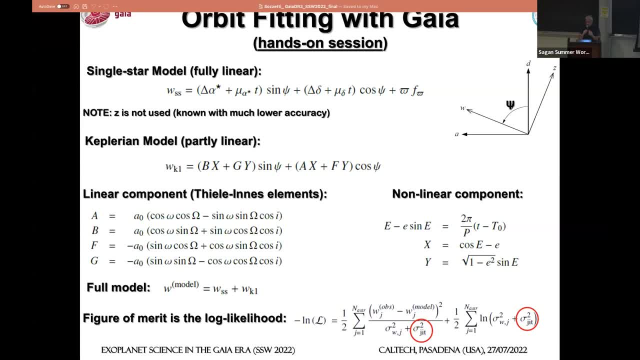 tried to challenge yourselves with the orbit fitting analysis you will not have to deal with, But we used it. It's what we called uncorrelated asthmatic jitter term that allowed us to capture essentially the gist of whatever we could not model as an orbit to identify. 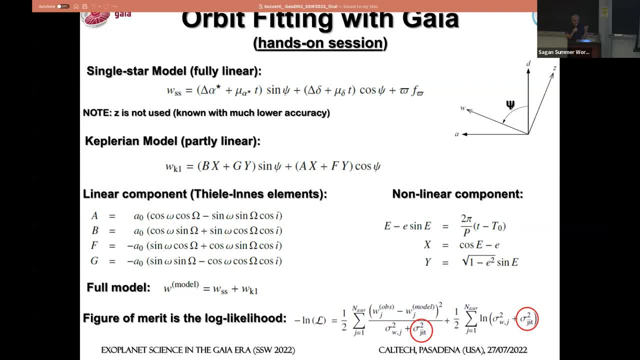 essentially the magnitude of the additional variability in the asthmatry that we cannot understand otherwise. To conclude, this is the Standard definition of a chi-square that I would like you to keep in mind because, again, in the hands-on session on orbit fitting. 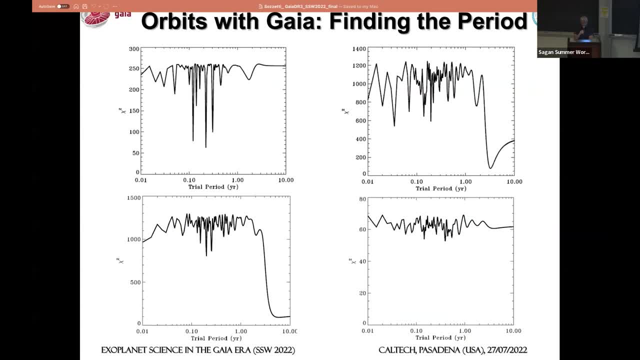 it's a quantity that you will have to play with. Something you will not have to play with but we had to deal with necessarily, was identifying first if there were significant periodicities in the data. And these are examples. These are examples through simulations, not actual data. 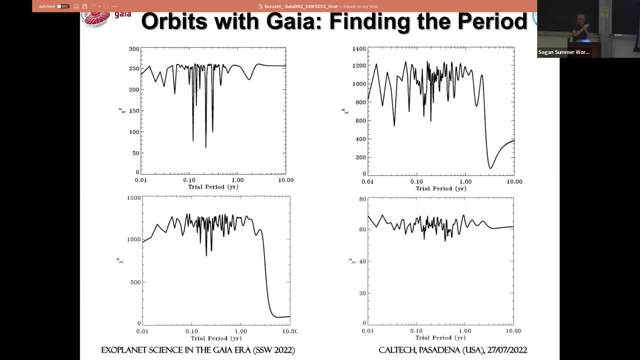 of how you can scan, Scan The grid of orbital periods for different configurations of orbits and find the one that minimizes the period that minimizes your chi-square. This is the quantity that allows you to identify a minimum corresponding to potentially a significant period in your data sets. 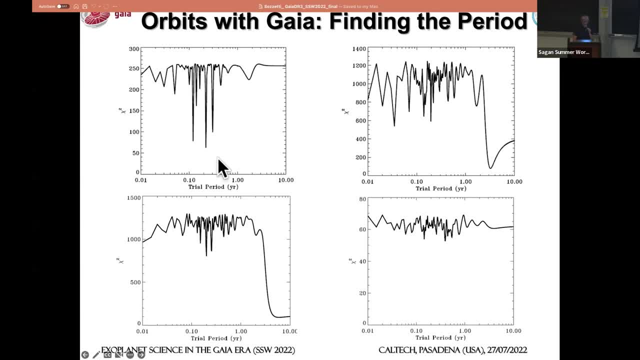 You see different cases, the cases of a very short period. object here: just a fraction of a year, maybe three, four years. a very long period: object: exceeding the time span of the observations And chi-square reaches a minimum but doesn't go, essentially remains flat afterwards. 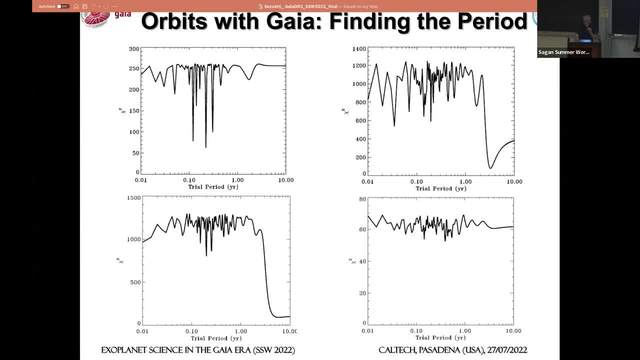 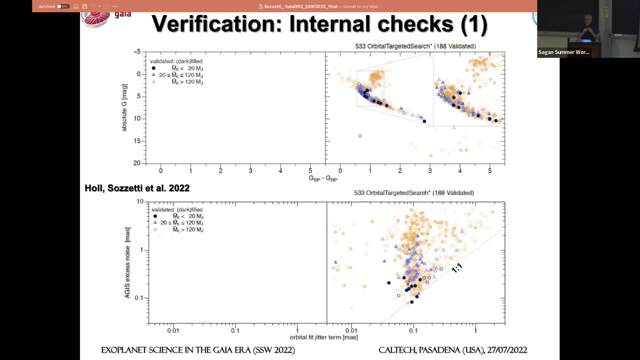 Or an object that doesn't show anything. There were many such instances in the sample we analyzed. When it comes to results, we had to deal with, as I said, many complications. We performed a variety Internal checks. Here there are two examples of what we looked at. 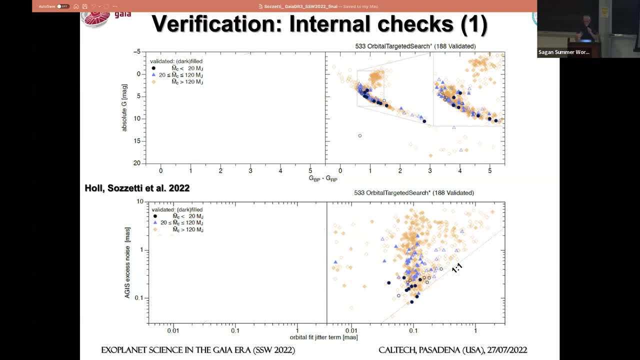 You are seeing in the right top plot orbits of companions characterized to be approximately, given the various symbols as planetary mass, Brandt-Wolfe, low mass, stellar, And you see them how they align on the HR diagram And the majority of these. 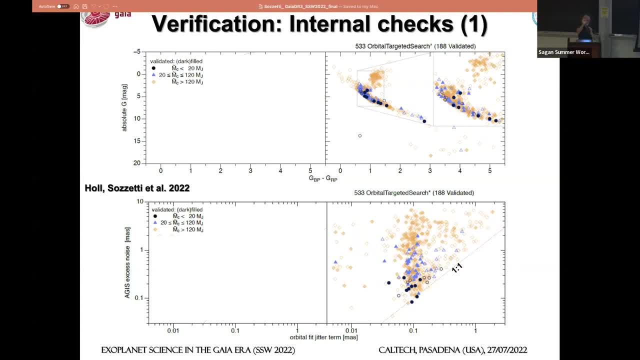 Indeed, align rather narrowly along the main sequence, Which is good, because we've already seen that if you have a large spread along the main sequence, that means that something bad is lurking. And another important point that we could use was in the comparison between our uncorrelated asthmatic jitter. 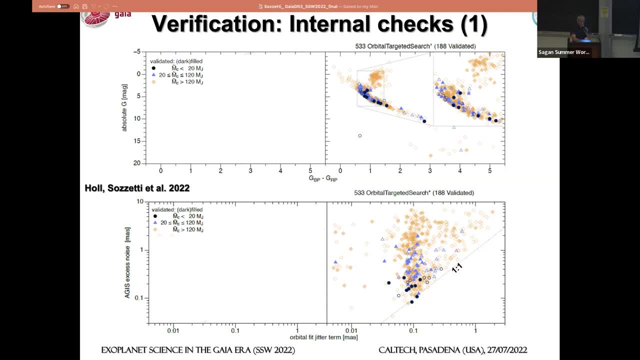 fitted in the model With the asthmatic excess noise value. that is also part of Gaia data release tree determined by the Aegis single star solution. Whenever we would get a very significant orbit, we would imagine that this jitter term would get much smaller. 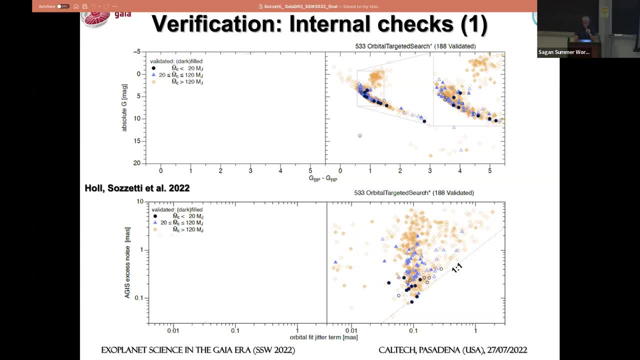 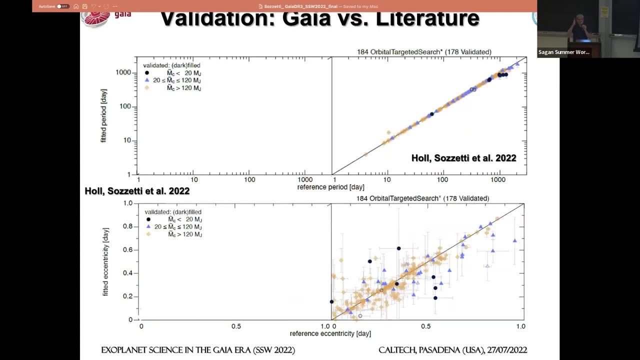 And indeed for many of these results, of these orbits. indeed, it is the case, as you see, in the bottom right panel. I think I can skip this one and go to the second step, After verification that the quality of the solution. 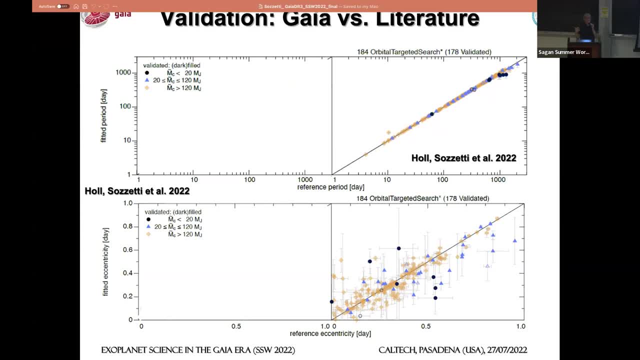 was intrinsically correct. we went out and checked that indeed, we had found something that was relevant by comparing with known orbital solutions from the literature. Here you see two examples of comparison: The orbital period in the top right panel, which actually aligns very, very nicely with the literature value. 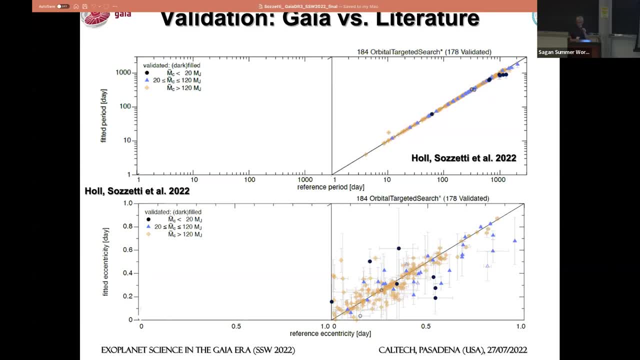 Gaia is the fitted period On the y-axis and the reference value from the literature is on the x-axis. There is only a small decrease in performance at the very end. As I had already pointed out, the very long period orbits tend to be underestimated in the value of the period. 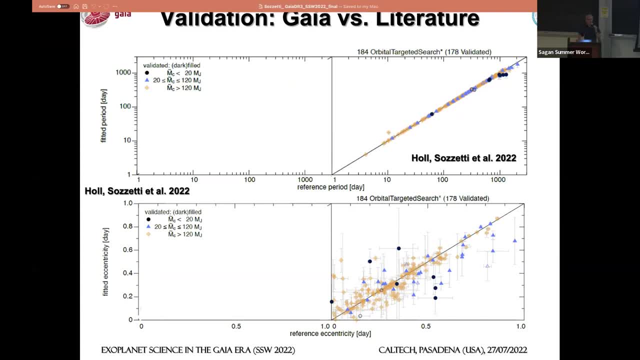 For eccentricity. things are not so good. They are approximately good, and this is also expected. The Gaia sampling is not very good, very high. The intrinsically one-dimensional nature of the observations doesn't allow for an extremely precise. 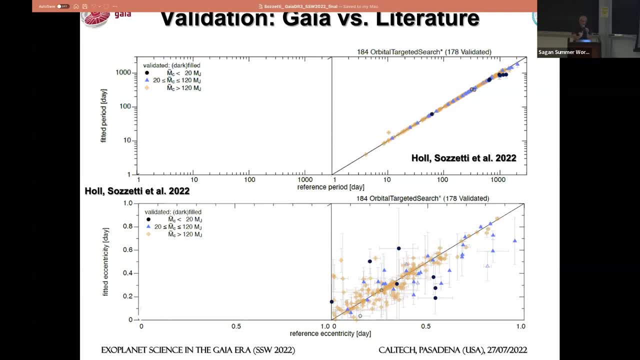 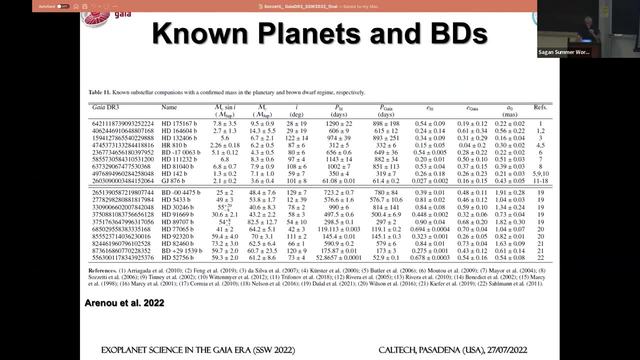 determination of the orbital eccentricities in the limit of Gaia-DR3 data set, which is still only a small fraction of the full one available, But nevertheless the correlation between the values, between literature and Gaia, fits reasonably good. Now to reach towards the conclusion. known planets and brown dwarfs. 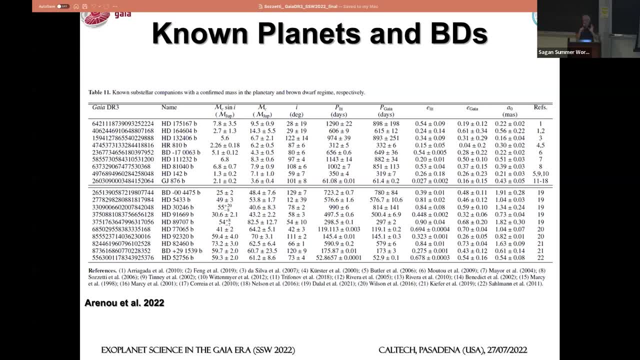 I mentioned, there is a small number of already known objects and I will briefly go through some of them to discuss them. The first thing I want to point to you is another somewhat element of complication. In this table you see the minimum mass of the companions. 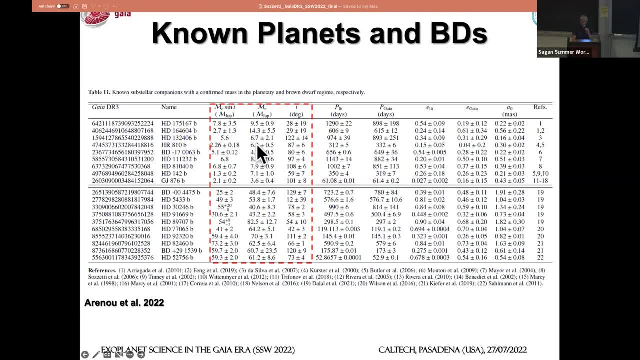 as it was determined by radial velocity. work, The true mass of the object inferred by Gaia and the inclination angle of the orbit as determined by Gaia. Mark my words: you don't have to do a calculation right now, As the minimum mass is mass of the companion times, the sign of the inclination angle. 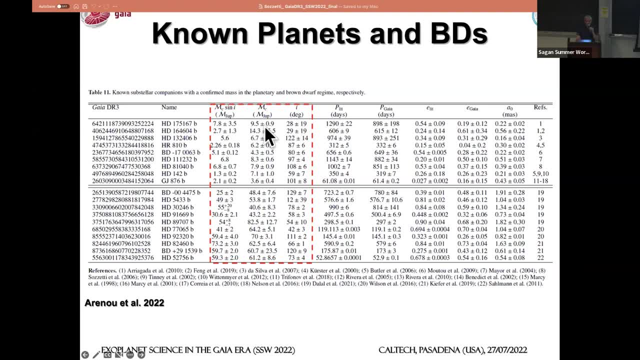 you would imagine that, given the inclination from Gaia, you can recover a true mass of the companion which is exactly scaled from the m sine i value For some of the objects here. this is not the case, So there is no direct mapping between these two numbers. 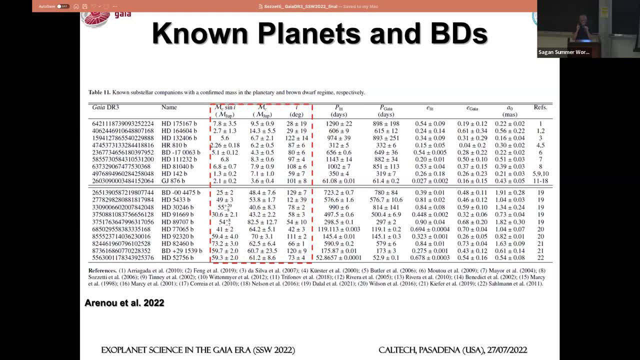 given the inclination measured by Gaia. This is an element of, let's say, of bias in the orbital solutions that we are aware of and we have underlined such that the companion is there. we have seen the effect, the orbit is determined, but not everything is 100% right. 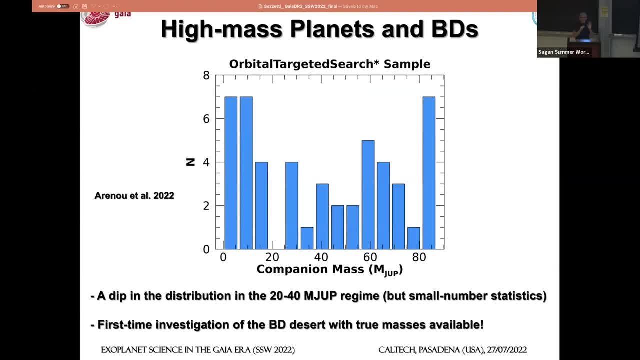 Even with small number statistics, one thing that we have been able to begin addressing again is the distribution of planetary, of boundary of masses, with true mass companions orbiting solar type stars. There is a very well understood, very well measured effect of decreasing frequency. 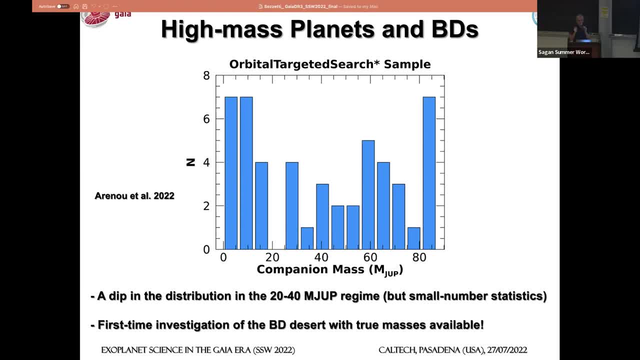 in the Brown-Dwarf regime with a minimum approximately around 20 to 40 Jupiter masses. This is a clear result that has been obtained through high-velocity work, In this case also with a true mass estimates from Gaia, we do see a hint of a potential dip in the mass distribution approximately around here. 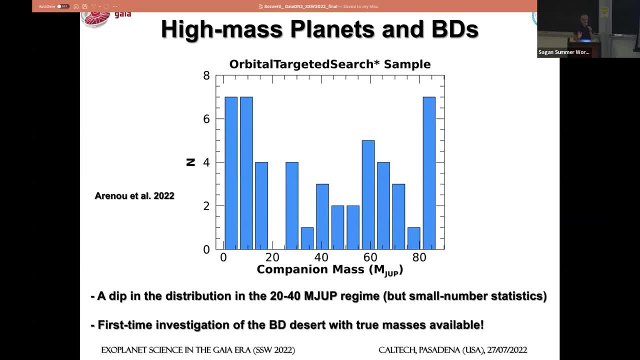 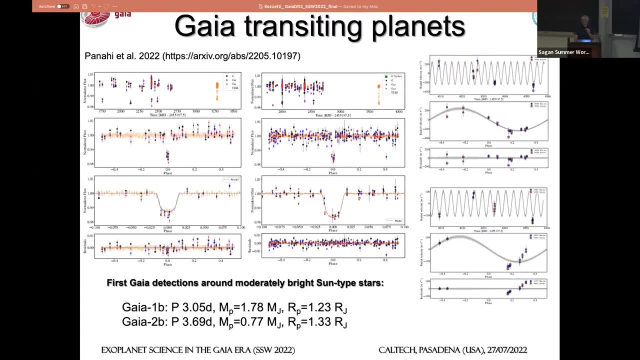 It is not statistically significant, but it is the first time that this investigation can be done with true masses available. I think I can skip the Gaia transiting planets that. we have already seen A few examples of DR3 astrometry at work. 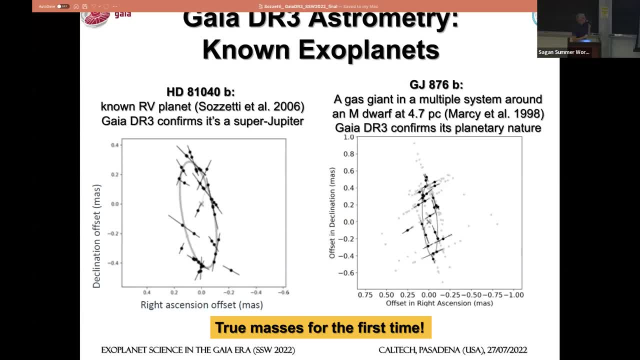 This is on the left is the orbit fit to a super Jupiter companion orbiting a relatively young star, HD 81040,, confirming that it is indeed a planet. This is just snippet of information for the hands-on session, if you decide to go through it. 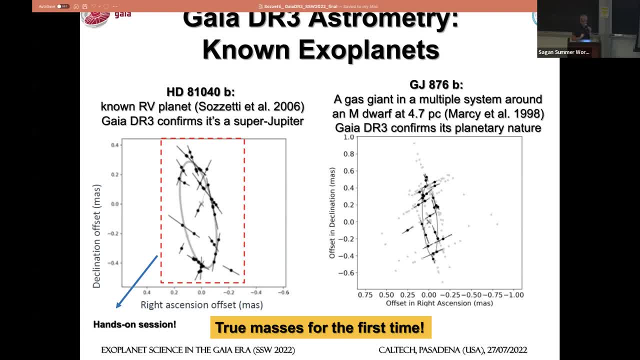 You will also be told or required or urged to try to plot the result of your orbit fitting. There is a non-trivial technique that you can try to use in order to actually over-plot to your fitted orbit in the plane of the sky. 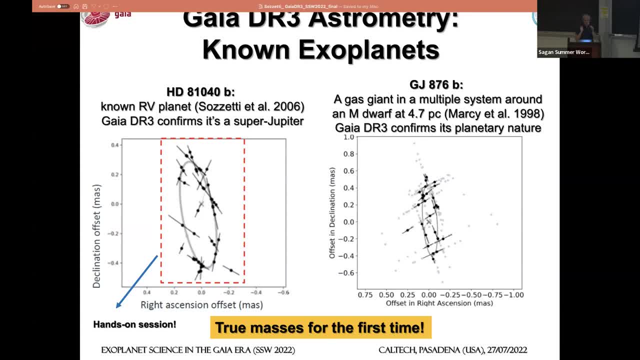 the Gaia data. We will get to this in the hands-on session On the right. instead, you have an example of a very good orbital fit to one of the very first giant planetary companions identified by Radar Velocity Worker all the way back in 1998,. 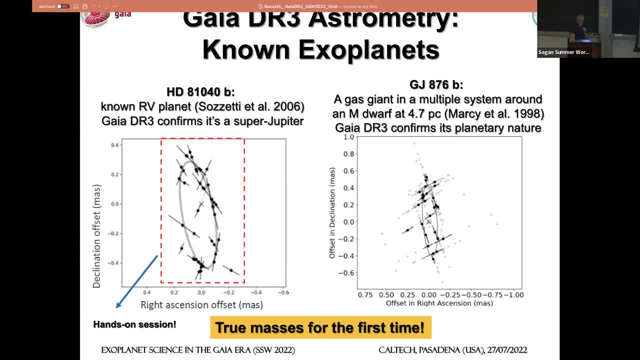 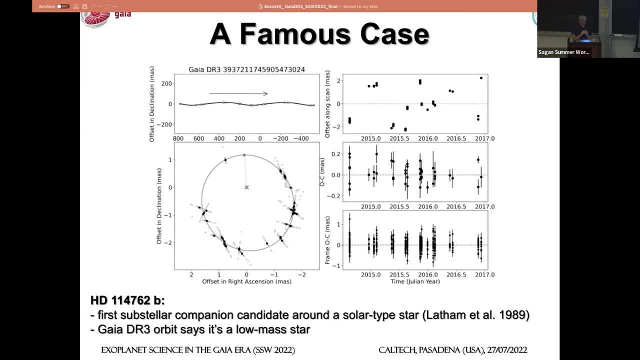 orbiting a very near volume: dwarf GJ876.. In this case- this is already underlined by others- a companion orbiting HD 114762b. This is famous because back in 1989, David Leighton and co-laborators had identified this companion. 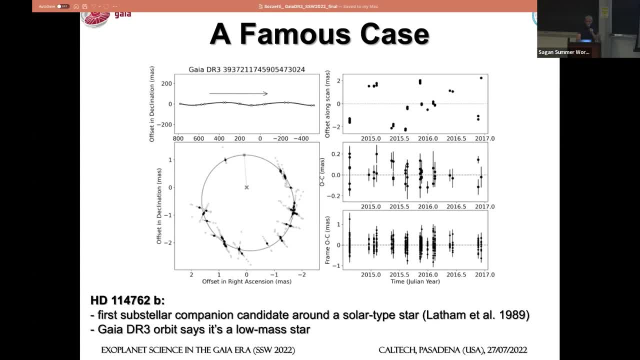 to be having a minimum mass of 11 Jupiter masses, and so it was the first potential planetary mass object identified. It had a minimum mass very close to the Brown-Groff regime, and indeed there were suspicions that it would be a Loma star. 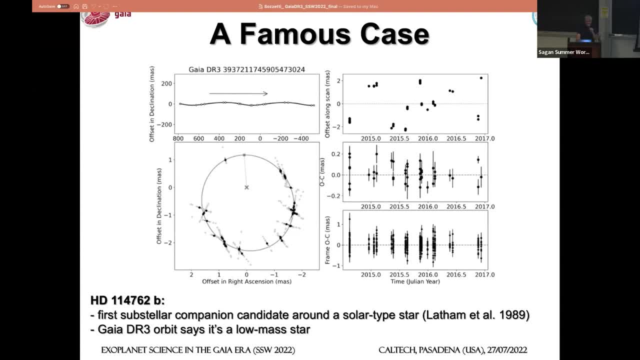 rather than a Mars star, But it was actually a Loma star, and the Gaia orbit that you see here, with a very large size of almost 2 milliac seconds, was entirely out of the planetary nature of the object. There are new candidates. 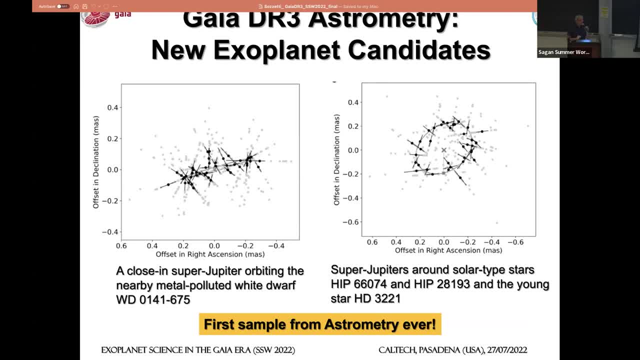 I show a couple of examples. On the left, a close-in Jupiter object, Jupiter mass object, super Jupiter mass object, orbiting a Vorb star. Remember some of the cases of impact on Gaia exoplanet science that I've shown at the very beginning. 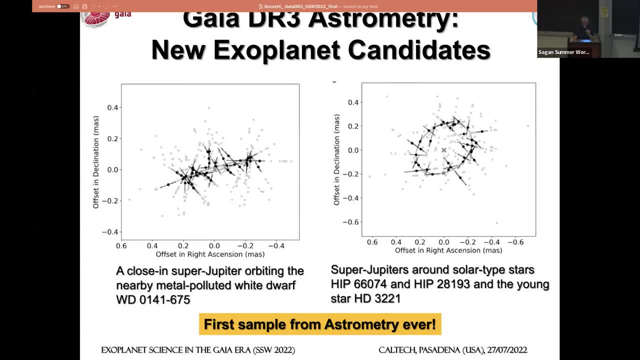 This is the first And on the right instead, the case of orbits of objects that were not known to be already there, And in some cases we have very good results. A few examples of these include Hipparchus 66074 or the very young star HD 3221.. 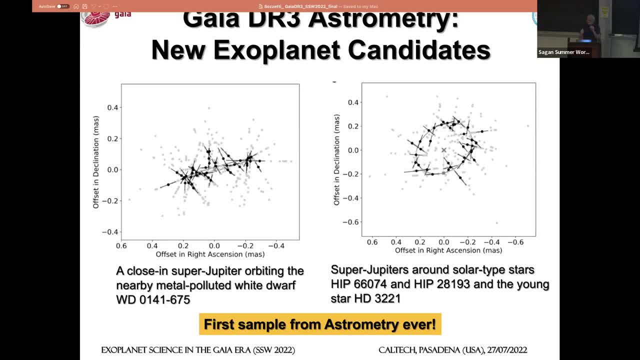 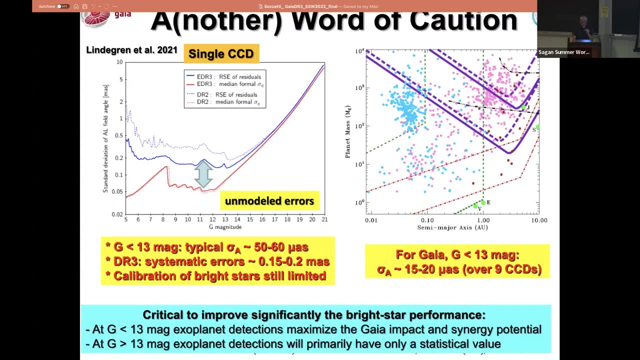 This sample, small as it may be, of order 70 or so, is the very first sample of planets candidates detected by astrometry. I will conclude with a word of caution: There is a lot of work to do. We have to do better than we have done so far. 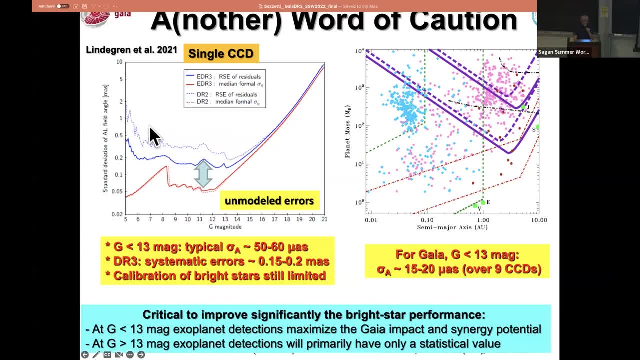 You see on the left diagram an improvement in terms of precision of the along-scan measurements at the single CCDE level from DR2 to DR3. This improvement that has diminished the impact of calibration errors, in particular in the bright star regime, is significant. 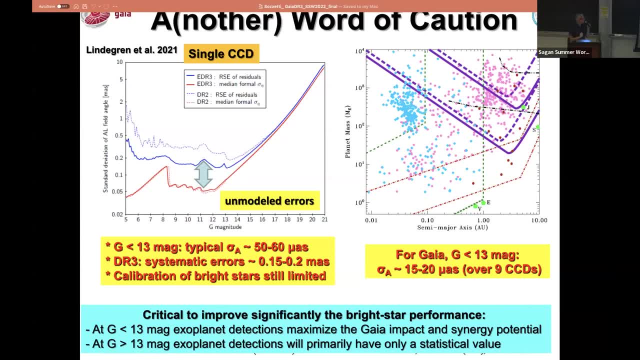 It's an improvement of maybe a factor of two and a half or so, But we're still a factor of three to four away from what we would like to really have. The bright stars are the golden sample for Gaia, for planet detection, because they are the ones that have the best chances. 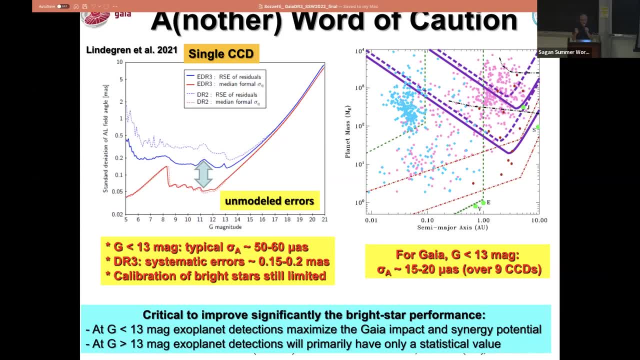 to be followed up by any other technique for improvement of the properties of the systems identified by Gaia and for additional studies, for searching for additional components and the likes. So this is really the task for the upcoming data releases: Improve the systematic floor, bring it down by another factor of three, maybe four. 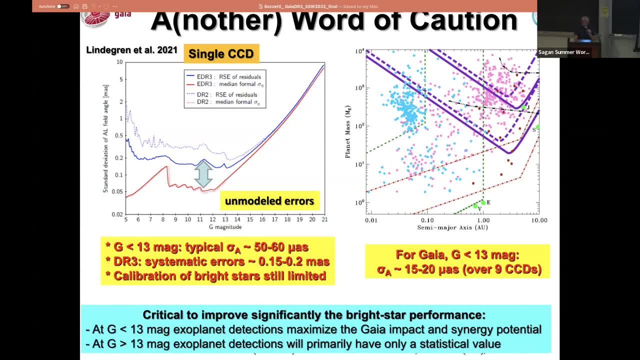 and ultimately achieve what we are really hoping to achieve. If this is the case and for the bright star sample we get down to where we hope to be, then I could say that I conclude with this slide. we will certainly be able to confirm. 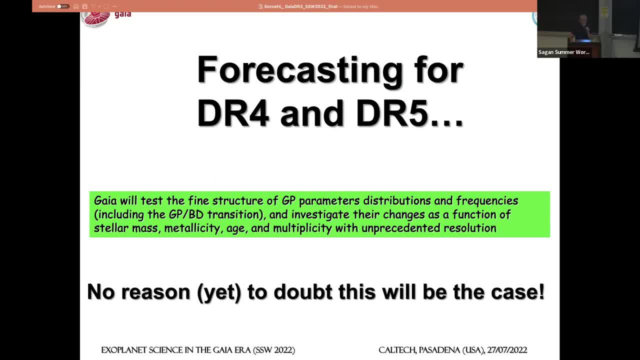 the estimates that have populated the literature in terms of Gaia yield for exoplanetary science, And I stop here After seeing you give versions of this talk about half a dozen times over the last decade. it is so wonderful to see actual planets in the talk. 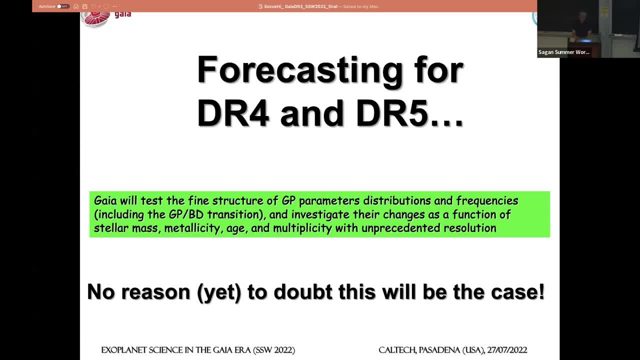 So it was fantastic to see. Let's see if we have a couple of questions here and then we can go to the ones online. Are there any questions in the audience here? Yep, Mike Alexandra, you've done so much, so quickly. 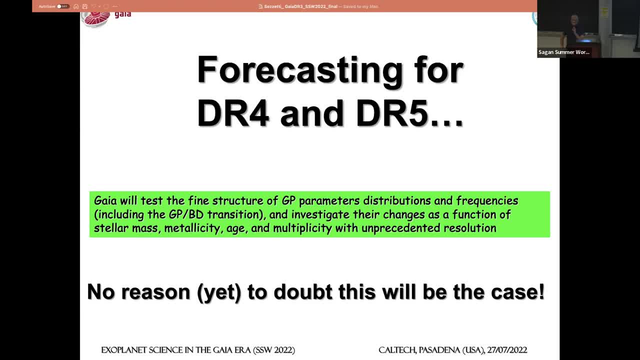 so I hesitate to ask for more details, but do you have any hints about the occurrence of two or more planetary systems, massive planetary systems? Can you just give us a feeling for how this is going to affect your detectability, your thresholds, your numbers and so on? 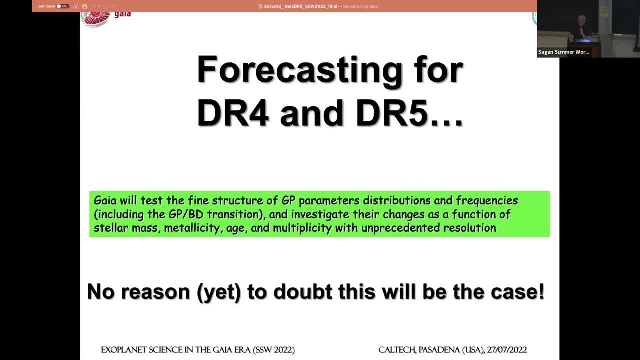 Obviously, it's another huge complication in the processing, but may I offer also my own congratulations on what this whole team has achieved so far. So we have done nothing in terms of searching for multiple companions with DR3. It was simply not possible for two reasons. 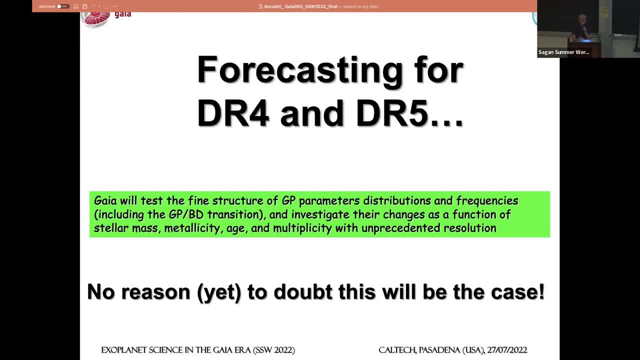 The first reason you have seen clearly explained that the data do not yet require allow for very deep investigations. The data set is too small and there are still insufficiently calibrated data sets for such investigations. Typically we have an order of 25 epochs. 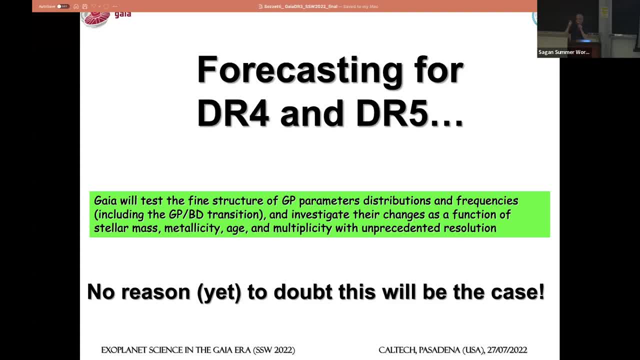 individual epochs in the sky and a model that tries to fit a second planet would have 21.. May I clarify my question? It's clear you don't have enough information to fit that multiple planet solution. My question was more: to what extent will the possible occurrence 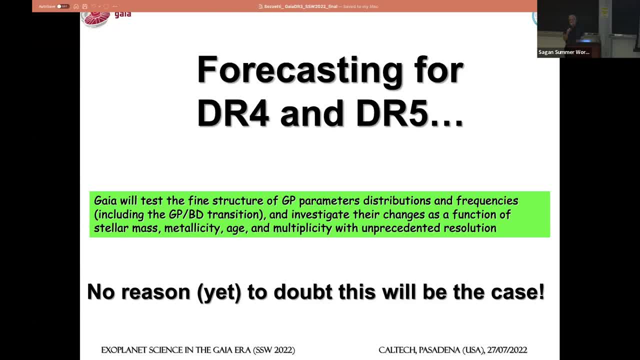 of multiple planet systems minimize or reduce the number of real candidates that you're able to search for. So you come up with a certain estimate of companion fractions. you know fractions, occurrences, but the presence of binary multiple planets will complicate that estimate. 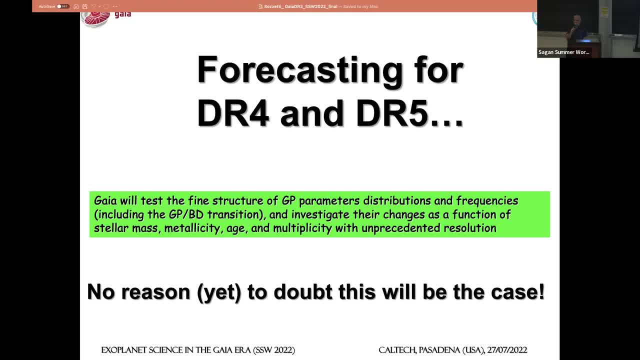 I certainly wasn't looking for multi-planet solutions at this stage For the present sample. any additional hints of companions that may pollute the data is very, very marginal for the present sample, The, For example, the case of GJ876b. 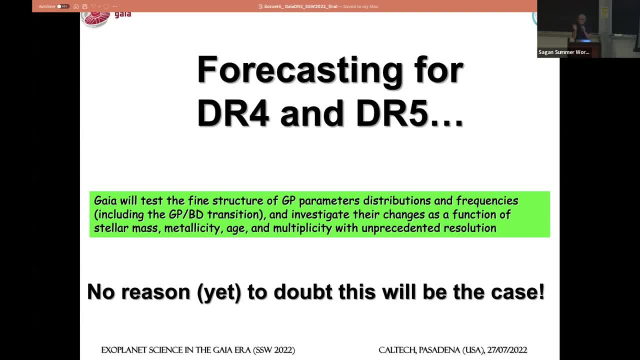 there is. The system has two Jupiter mass objects on a two-to-one resonance. The one we see clearly has a 60-day period. There is one at 30-day period. The one at 30-day period has a much smaller asthmatic signal. 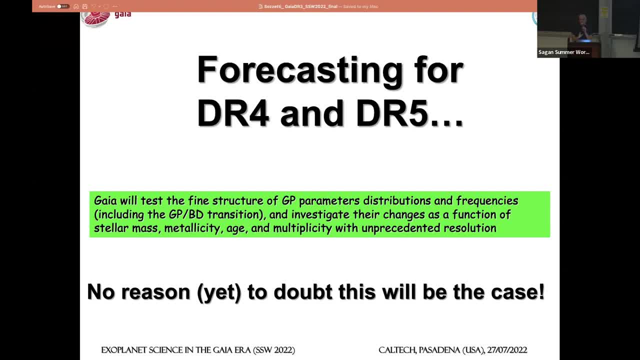 and so it doesn't impact at all the measurement of the orbit of GJ876b In the long period regime. the typical architecture of multiple systems that we see from radio velocity surveys looks at systems that are very widely separated in period duration, So the ones that we see at 1,000 days. 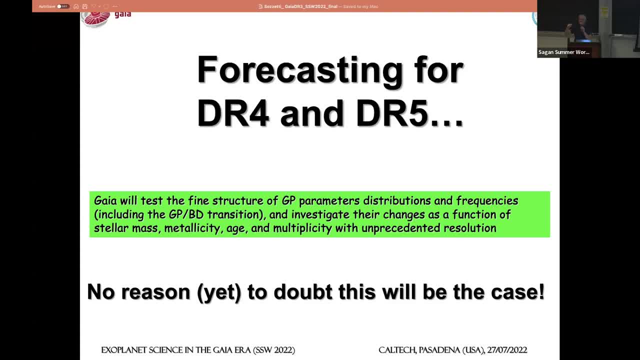 there is nothing expected to be there at 1,200 days, And so having covered the full cycle of the inner component essentially still tells you very little about any outer components. So from this point of view, it is not. It is not, let's say. 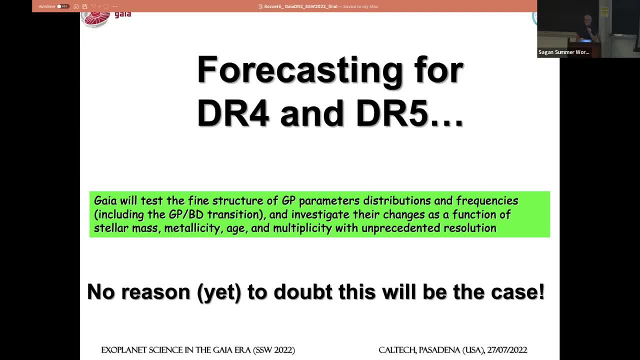 a big bias at all: the presence of multiples. We will have to deal with that as soon as we have six and a half years of data available. Two more questions in here. Please identify yourself, and then we'd like to get to some questions online. 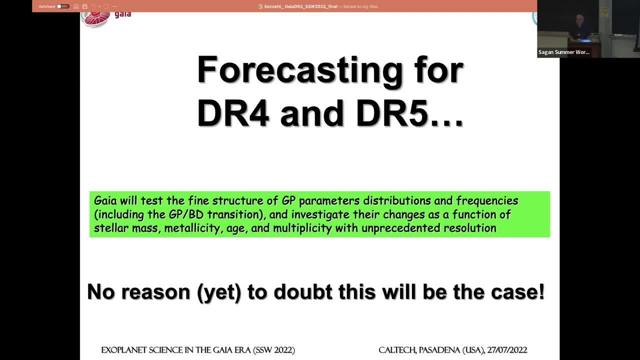 Good talk. Thank you, Hi. I'm Dom from the University of New Mexico. One thing that intrigued me about these results was the scatterplot of companion mass against stellar mass. It showed, Or it seemed like you had a lot of brown dwarf candidates. 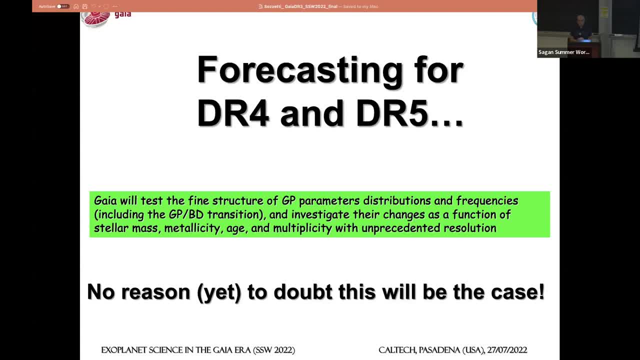 or brown dwarfs around M, dwarfs like lower-mass stars, And I'm wondering if you could kind of highlight implications for formation in those systems, because that seems pretty interesting. This is the To do this right. you have to have a good sense. 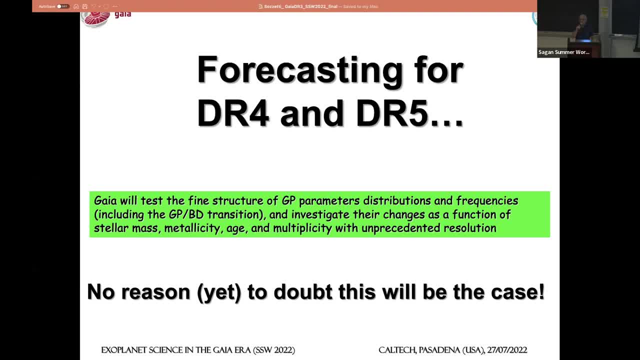 of the completeness and reliability of the survey. The numbers that I quoted, for example the rough estimate or potential occurrence of these objects around the low-mass star sample, is significantly underestimated. So until we have a good sense of how incomplete and how reliable the results are, 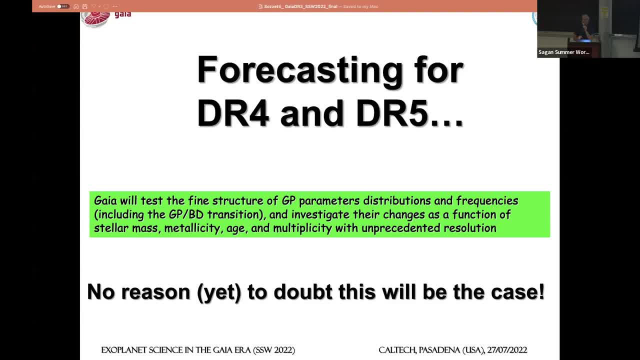 it is difficult to tackle the question that you have put forth, But this is definitely something that will be done because it's a key. Once you have the right number, then you can elaborate and say why this and how come they have come about and they have formed. 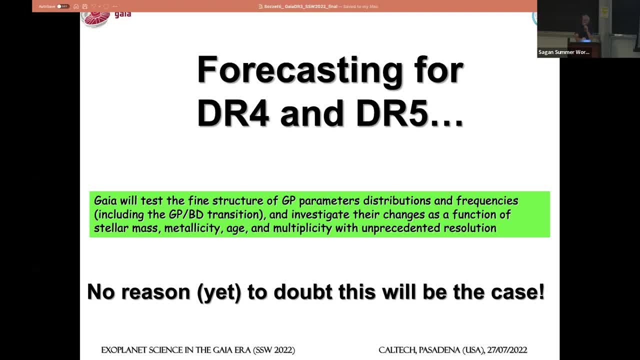 The number right now is smallish, but it's certainly larger than the one we quoted, because we are certainly very incomplete And if it becomes over the 1%, for example, this number is ballpark, the same as the one that has been estimated for larger mass stars. 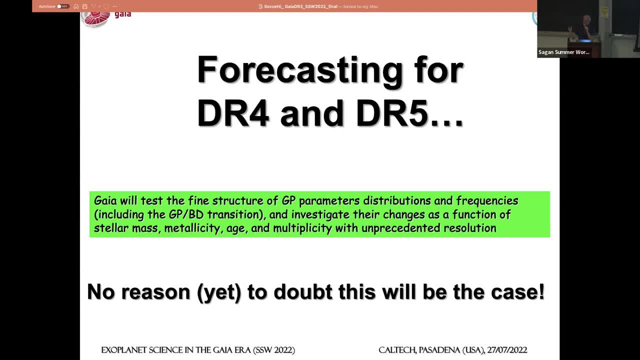 The Brown-Dwarf frequency around F, G and K-type dwarfs is already rather well established through high-velocity surveys and that number is over the 1%. So if the N dwarfs end up having the same number or they don't get the same number, 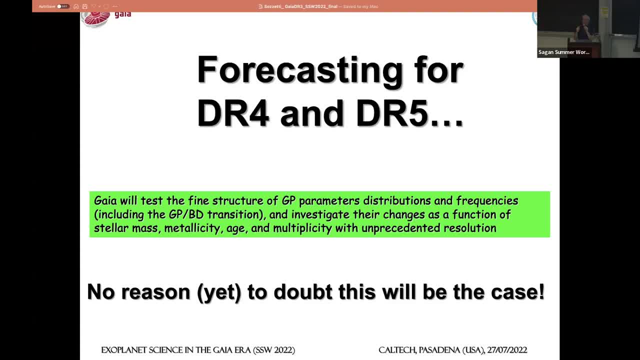 that tells you something about the formation, But it is still preliminary to make any extrapolation, but we still have to do the first exercise, Thank you, Thank you very much everyone. Hi, Orla Creevey, from Nice, First of all. 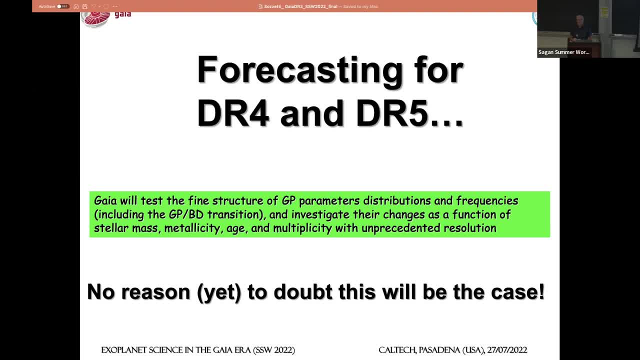 thank you very much for this really amazing work that you've done. I don't actually have a question, I just have a comment, because you have an element of you know: be careful with the data. There's things in there and I think it's. 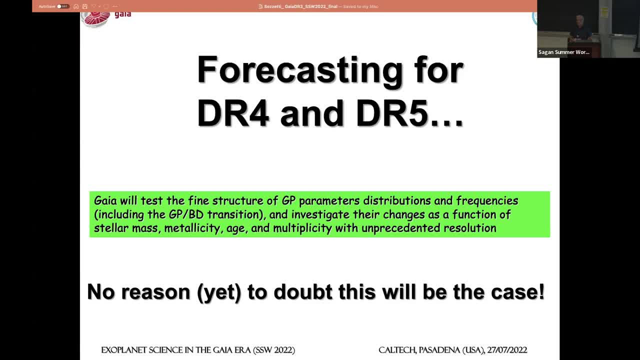 a very, very important point to make. if you put out things that you know just for certain, We're not going to learn anything right. There's a huge astronomical community out there, lots of tools and lots of other ways to investigate things, so this- these have to go out as well. 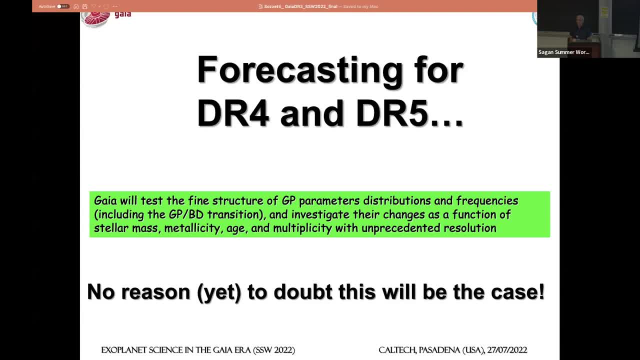 because you will only get much better by getting their feedback right. so, while it's important to make the point, be careful, it has to go out, like you know, absolutely. in fact, I I don't say I'm unhappy of having done this. the, the, the, as long as we identify the things that are still not. 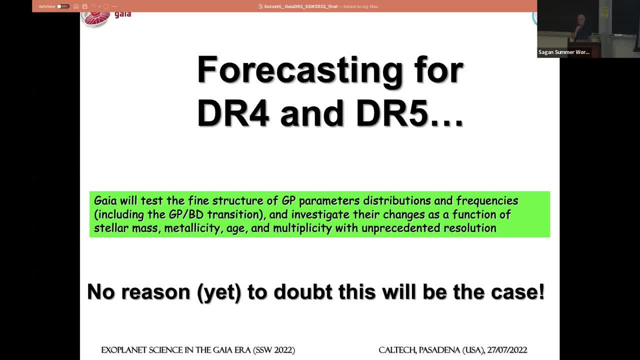 working and we, we make it clear to the, to the, to the community, that nothing is perfect. there are still things that are, that are murky, but we understand why things are like this. then we say it, and this is exactly what we always try to do: yeah, okay, uh, maybe we've got time. 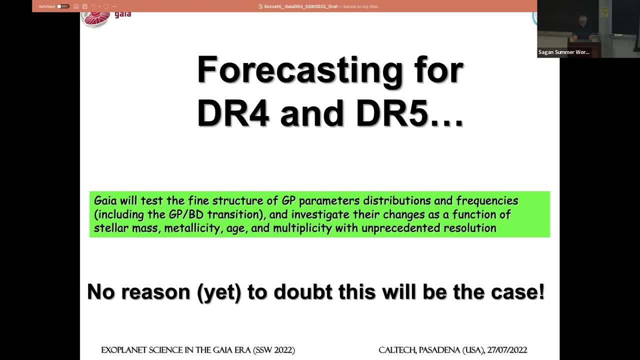 for one question online. we're running a little bit behind, all right. so, uh, one online question: how many explained candidates are expected in the next Gaia data release- $50 million- question, which I can reply. if everything goes right, then the this number of 70 that you're seeing here is gonna get much bigger, but I'm not sure I want to give a number now.